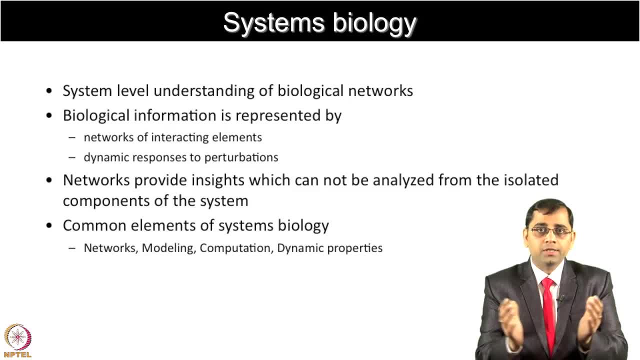 and try to obtain the full picture. We have to start putting the things together in a more systems wide manner which could be analyzed using systems level tools. So what are the common elements of system biology? They include the networks, modeling, computation and dynamic. 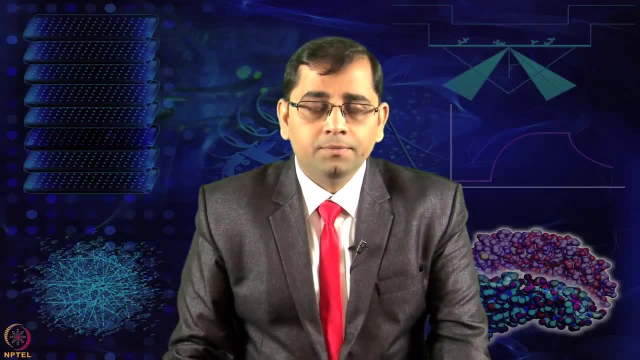 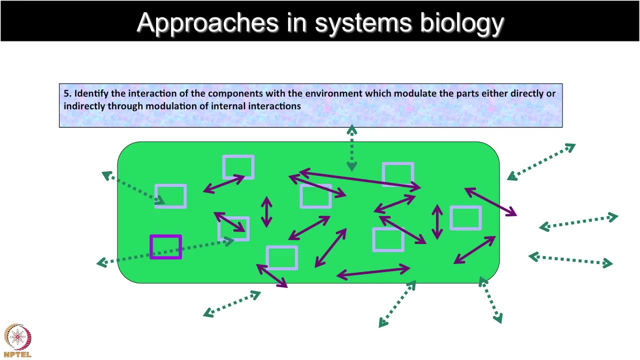 properties. So what are the approaches of system biology? The system is an entity which maintains its existence Through mutual interaction of its constituent parts. You can see at the side that system research consists of first identification of the parts, then characterization of these. 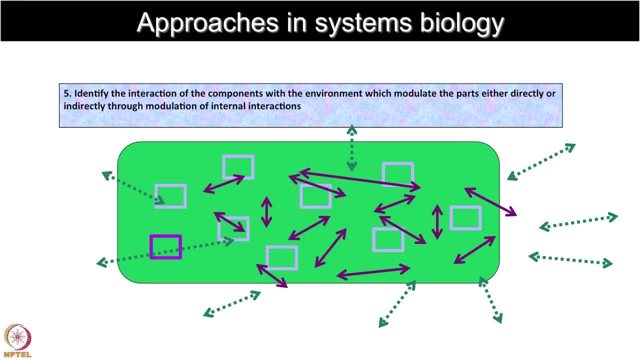 components, excluding the ones which are not the part of a system, and then identifying the interaction of the components with each other. Finally, we are looking at the interaction of these components with environment, which modulates the parts, either directly or indirectly, through modulation of these internal 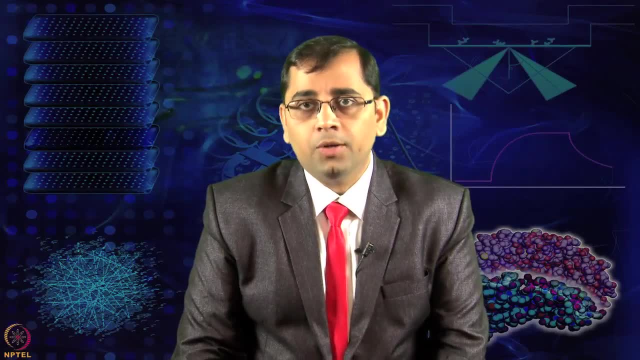 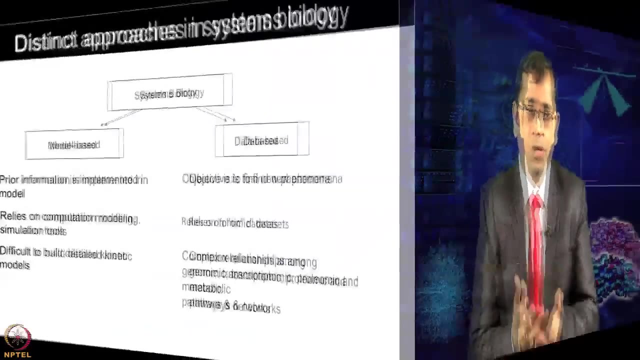 interactions. So what are distinct approaches in system biology? It can be model based or data based. The model based: you already have the prior data information which you want to implement and build the model. Of course it relies on lot of computational. 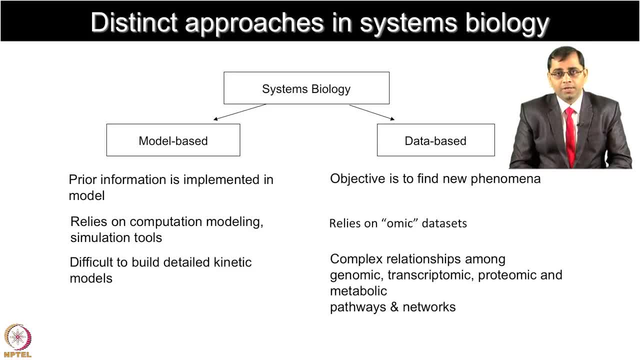 modeling and various type of tools for simulation, but it is very difficult to build the detailed kinetic models just based on this information, Whereas the data based system, biology and biology approach involves a new phenomenon to define or find using these kind of you know datasets, It relies essentially on various type of omic datasets and looks at their intricate 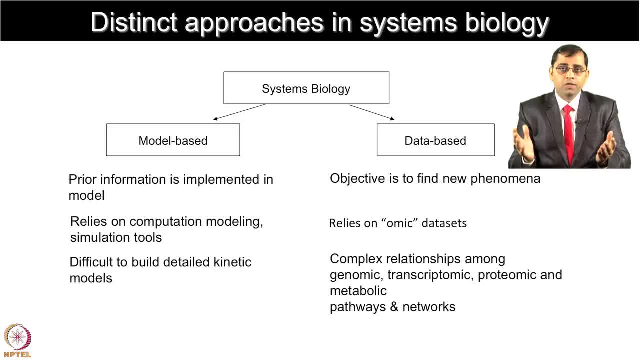 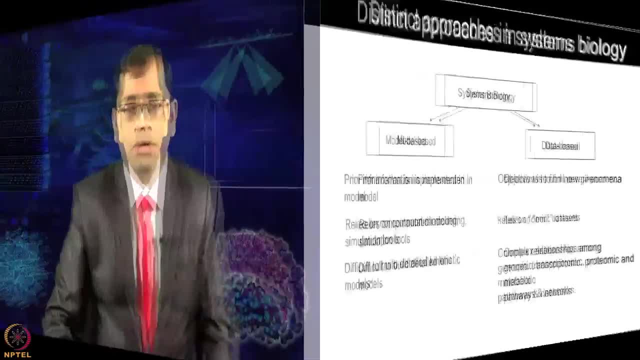 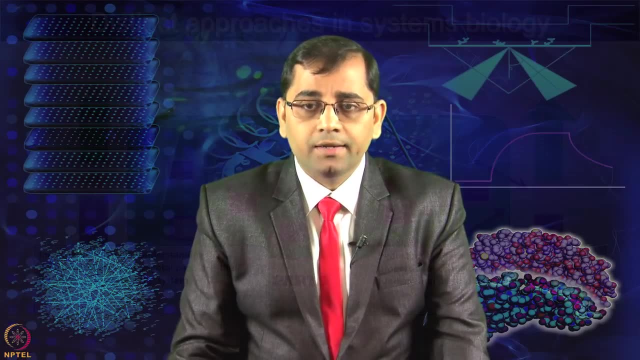 complex relationship by looking at various components from genome, transcriptome, proteome, and then try to define various type of pathways and networks. There could be different ways of looking at the system biology approaches. One is reductionist approach, which is understanding the properties of complex systems by studying their fundamental 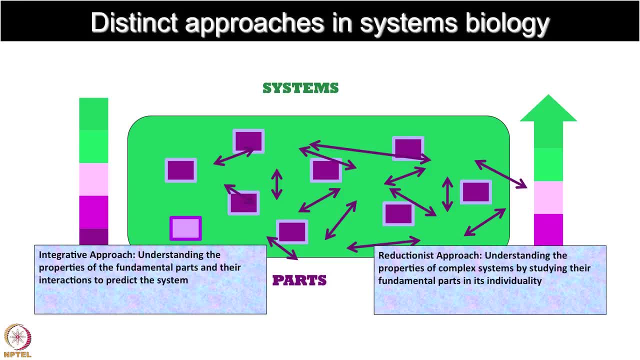 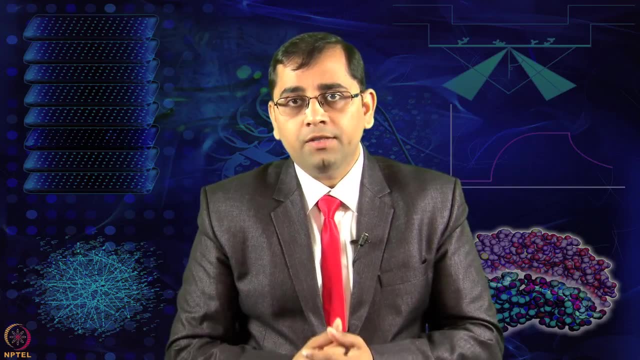 parts in its individuality, or it can be integrative approach where we want to understand the properties of the fundamental parts and their interactions to predict the system. What is system biology triangle? It involves the experiment which we do in the wet lab to generate the data set, the various technology platforms and computational models. So we 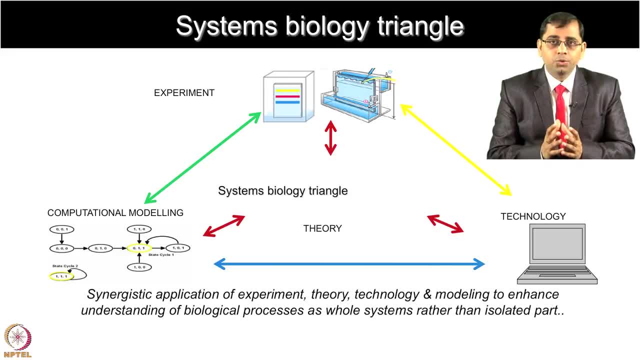 call it system modeling. All this together constitutes the system biology triangle. This is essentially the synergistic application of experiment theory, technology and modeling to enhance our understanding of the biological processes as a whole system rather than looking them as the individual components. So I must warn you that system biology field is very 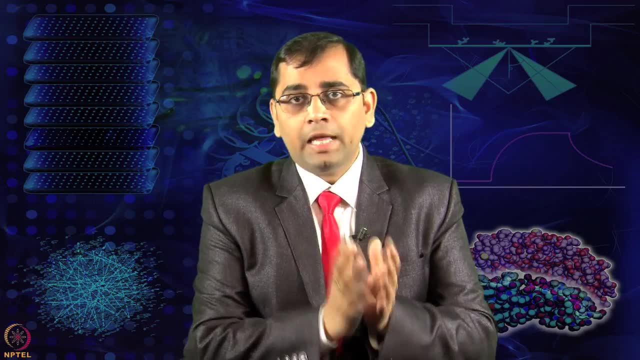 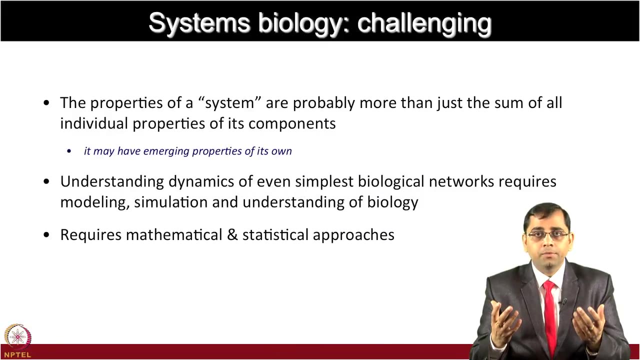 challenging because you are looking at not only one type of data set in isolation, but you are trying to integrate the information and looking at the properties of a system in its whole, which is not just, you know, simply adding 1,, 2, 3 and making the sum of that. 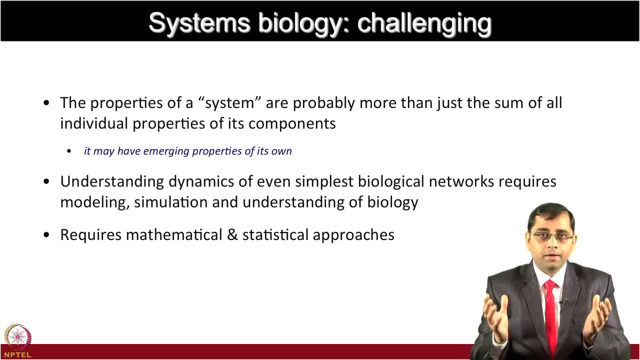 but looking at much more bigger picture and trying to integrate the information in much more meaningful manner. And when you do systems analysis, you might find out that system may have its own emerging property on its own, which was not just possible by looking at each pieces separately and just. 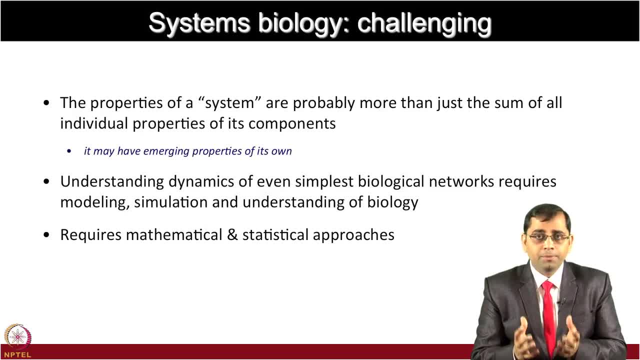 by combining them together, Understanding the dynamics of even simplest biological networks. it requires lot of computational power, using modeling, simulation and understanding of the biological questions. It also requires mathematical modeling and different type of statistical approaches. I have depicted you here the one of the omics data set obtained. 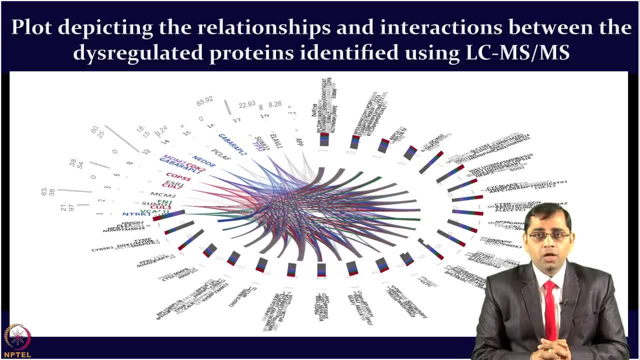 from the microarrays and mass spectrometer And then how we were trying to build the interaction networks of various proteins which were in the system. So by looking at this kind of information we want to really obtain what are the important nodes which might be governing the disease, which was otherwise not possible just by looking. 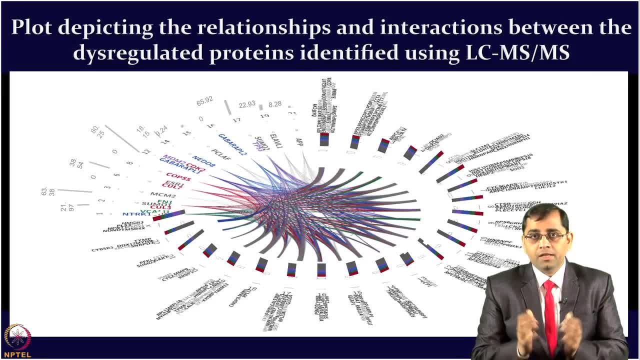 at the list of the protein and what kind of proteins are changing, but rather now we are comprehensively analyzing the entire data set and looking at which could be the major root cause of the disease and can we identify the right nodes. If we identify those, the 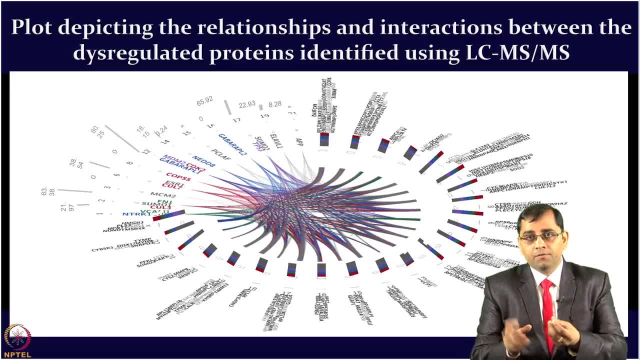 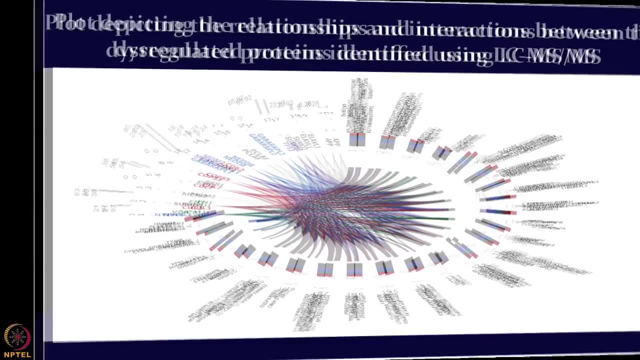 major area. then of course one could think about certain therapies which could target those nodes, and then probably those will be the root cause where one could start making more impact for the patient treatment. So in my next part I am going to now talk to you about some of the major revolutions. 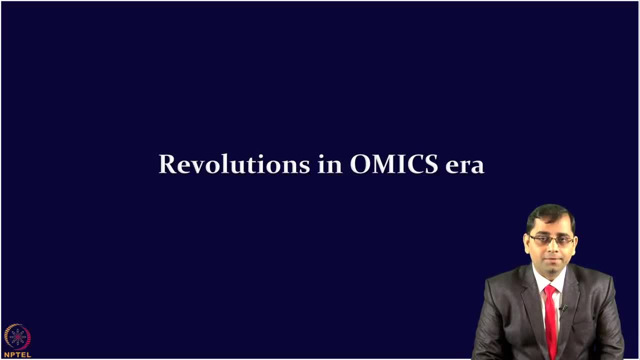 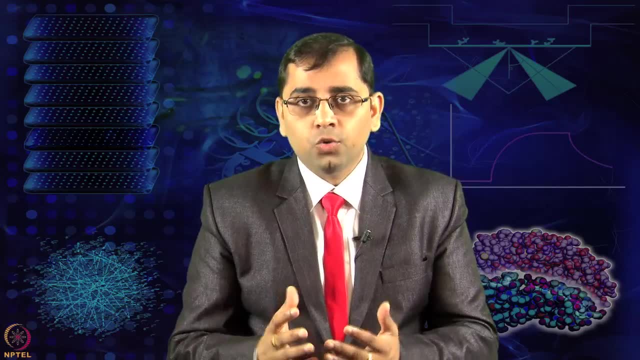 which are happening in front of us in the field of omics. I am going to give you some very brief examples and also going to give the perspective directly from the experts, the scientists who are working on this field and who have actually laid the foundation. 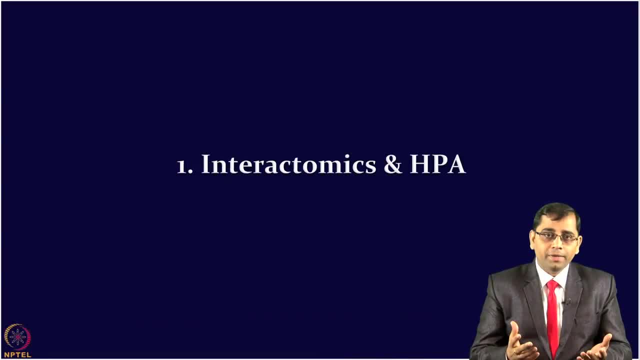 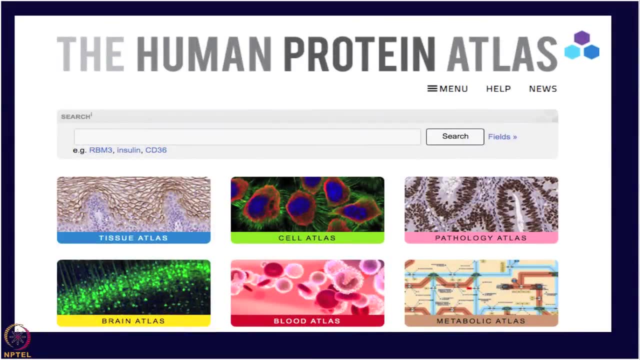 for these areas. So first, in the field of interactomics, The big project has come forward which is the human protein atlas, The scientist Mathias Ulhan and his big team. they are all working towards generating antibodies for each protein and looking at that, how the proteins are localized, how proteins interact and they are providing. 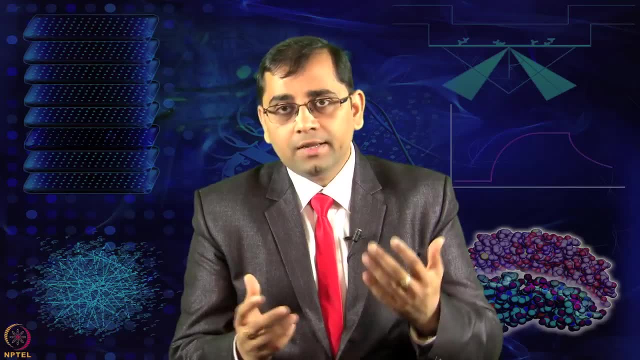 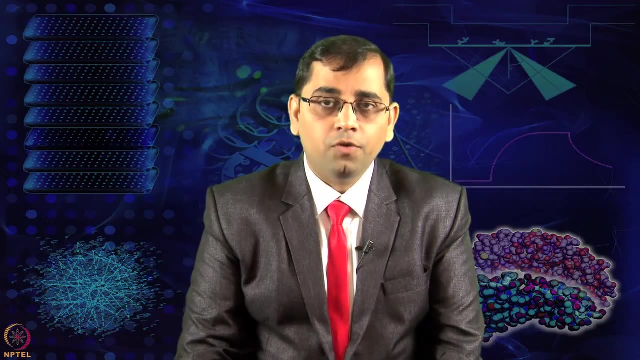 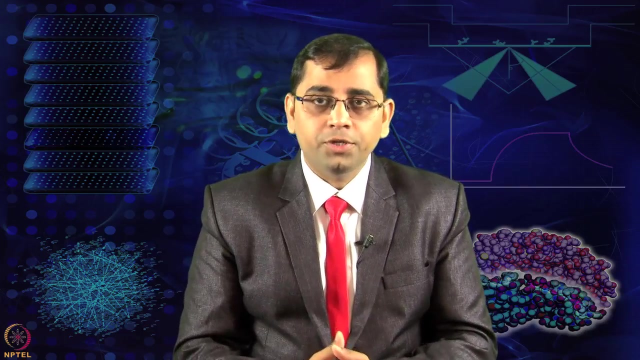 lot of interesting biological insight looking at the proteins by different type of experiments which are based on the antibodies. So let me have a perspective of Dr Mathias Ulhan- Mathias Ulhan and Dr Emma to talk to you about what are the goals of this big project. 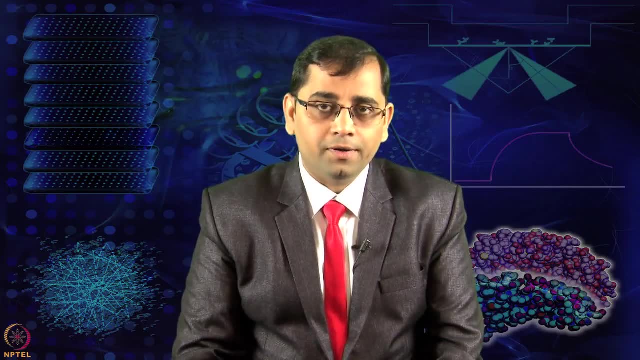 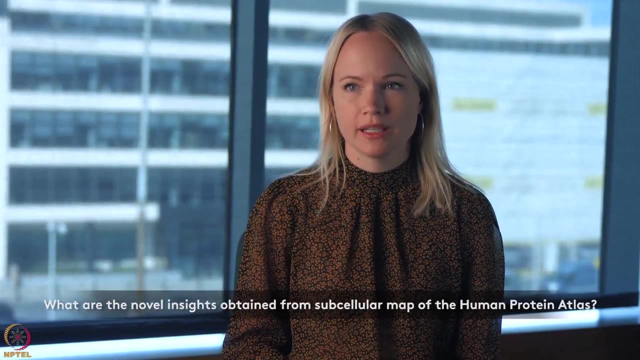 of human protein atlas and what are the major accomplishments so far? So we have, during the last 10 years, as part of the human protein atlas project, we have been making a cell atlas, a subcellular map of the human proteome, using an antibody based. 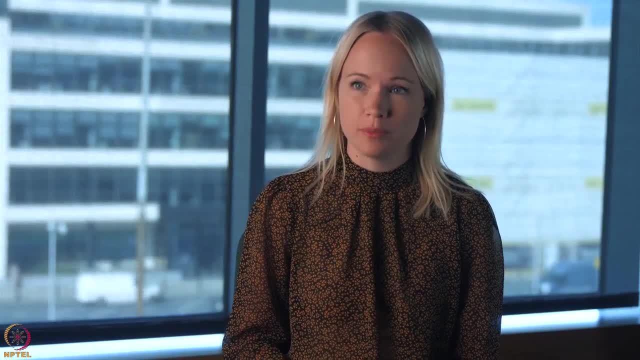 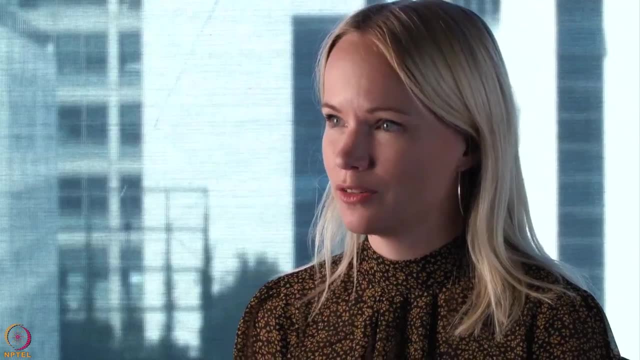 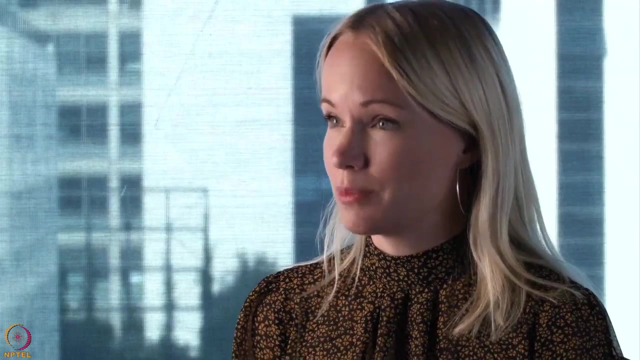 approach, So we generate high resolution fluorescent images and we have been generating hundreds of thousands of such images. And then we have been creating a cell atlas, So we have been classifying the patterns and sorting it into different categories so we could finally provide the first map of the first subcellular map of the human proteome. 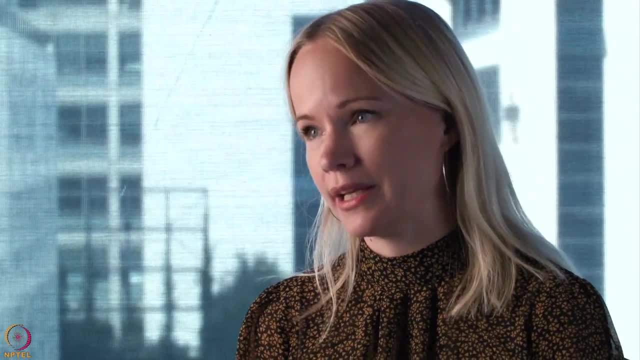 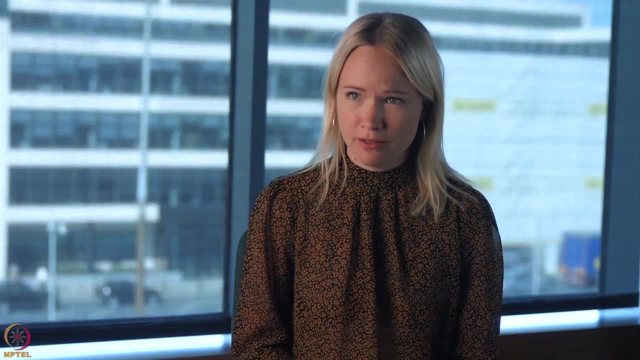 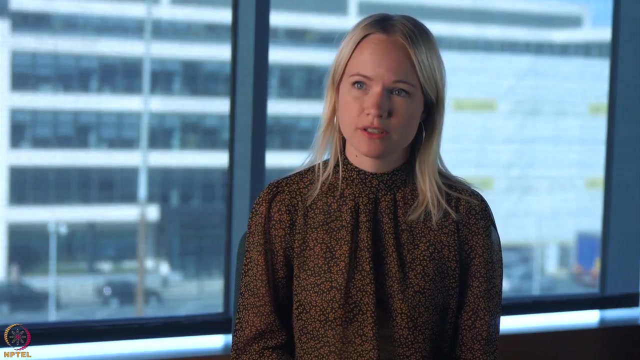 and see which proteins are in the mitochondria, which proteins are on the plasma membrane and so on. And the most interesting findings we made here is that as much as half of all proteins localized to several places in the cell and we also see a lot of single cell variations. 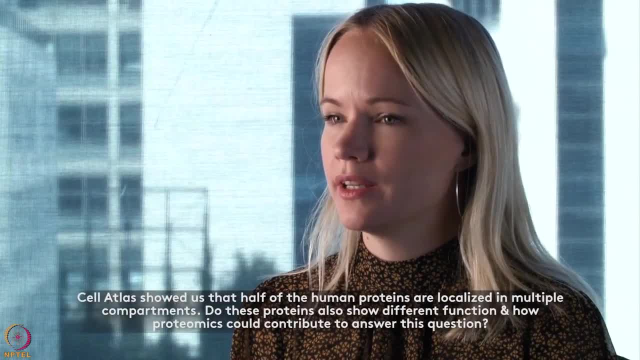 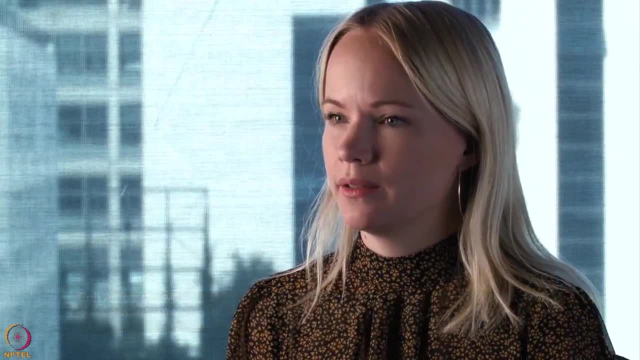 So the multi-localizing, So the multi-localizing, So the multi-localizing proteins as we call them. it's very interesting from a biological perspective. We don't know the biological consequences of this. It might be so that these proteins have context specific functions or even moonlight in different. 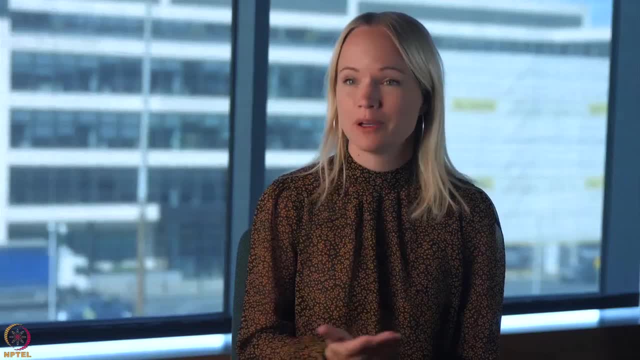 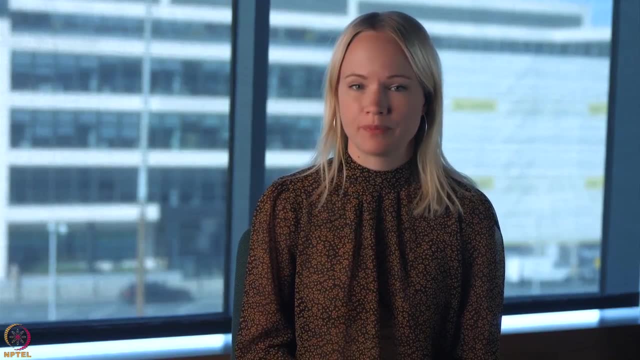 parts of the cell, but we can't really tell. We can only observe, make the observation that they are in multiple places, And then someone else would have to do in-depth biological studies. look at splicing isoforms or post-translations. 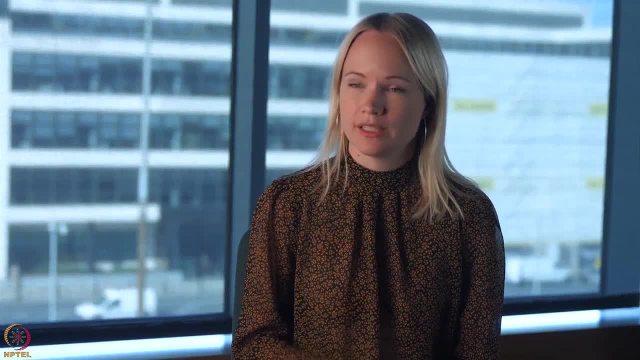 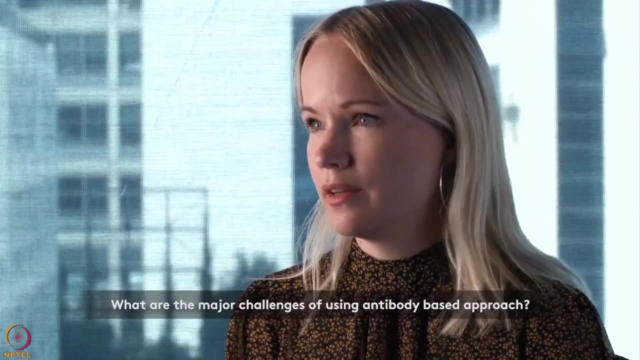 So we have to do a lot of biological modifications to see if it's how this multi-localization is achieved and also what the biological consequence is. My opinion is that antibodies should be viewed upon as small chemical reagents. They have on and off target binding, so you have to validate your results in any assay. 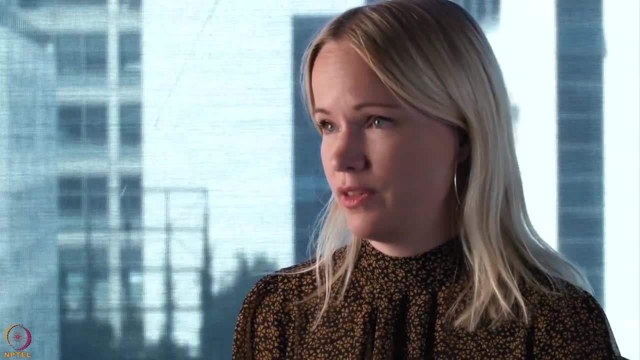 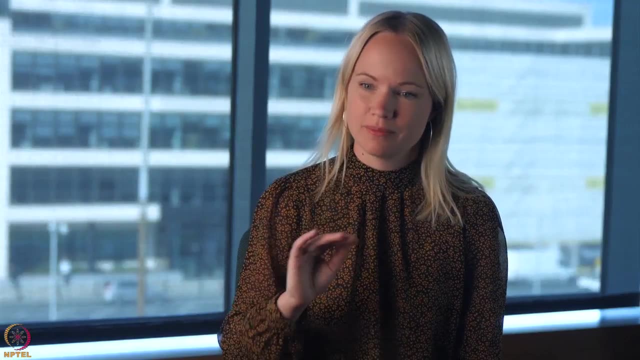 where you use them. So we fail more than half of the antibodies that we use. so we put a lot of effort into validation of our data And we have validation scores that kind of denotes the reliability of the results. So we put a lot of effort into validation of our data. 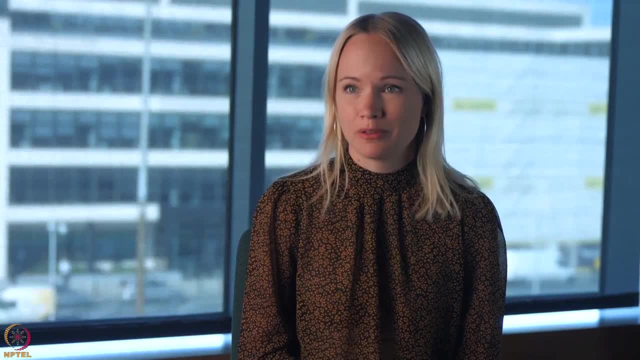 And we have validation scores that kind of denotes the reliability of the results. So we put a lot of effort into validation of our data. So that is the big part of our job. Next, I'd like to talk to you about the field of proteogenomics. 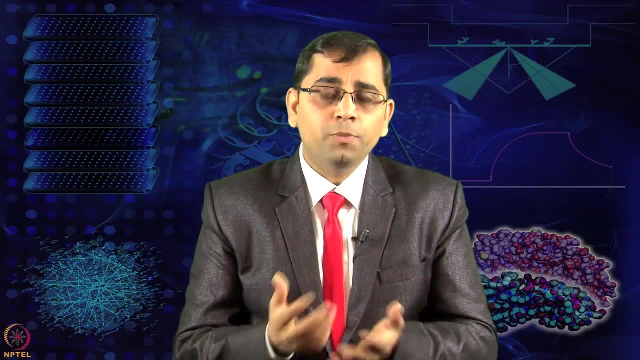 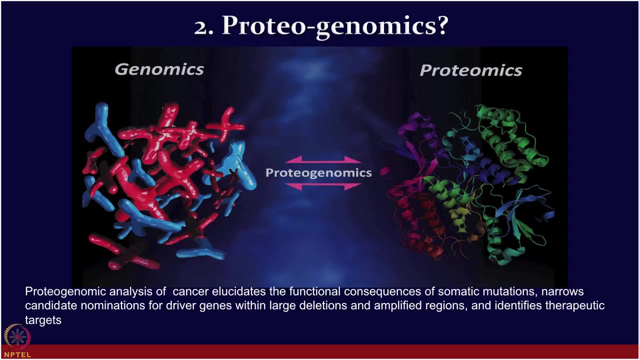 By a lot of things. we talked about different proteomic technologies, but you have also seen that how NGS is contributing. next generation sequencing and genomic field is contributing immensely towards our understanding of the biology. So how to integrate this information? Can we start integrating the most crucial molecules, the genome and proteome together? 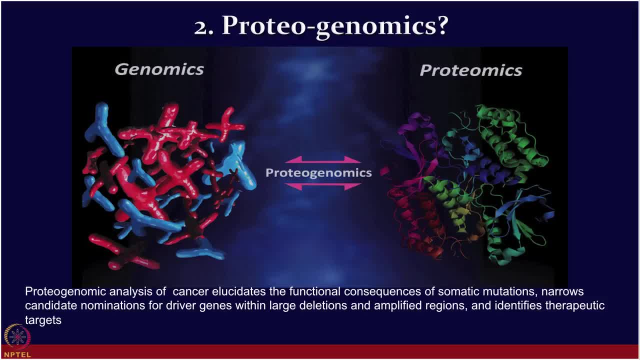 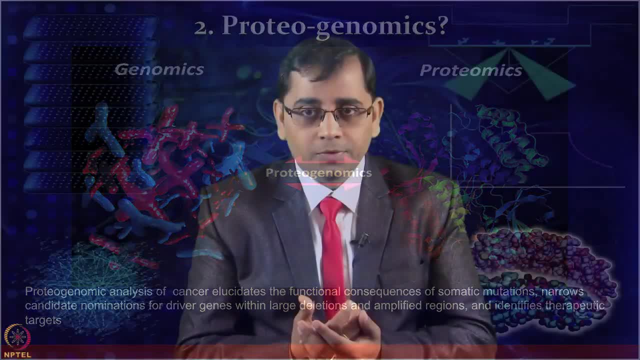 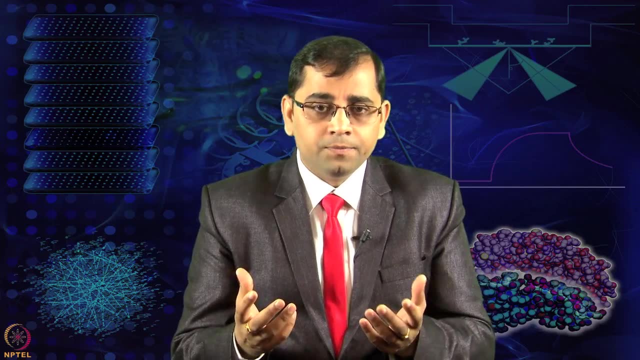 And that has actually led to the field of proteogenomics which is essentially going to look at, you know, lot of information which was not possible otherwise by looking at the molecules alone. Probably with this cartoon you will appreciate that how the proteogenomic analysis of cancer and other complex diseases could elucidate the 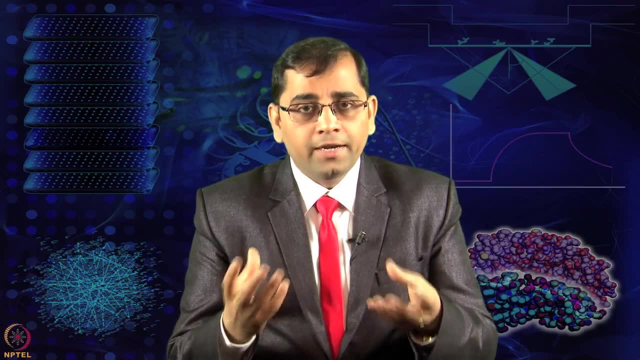 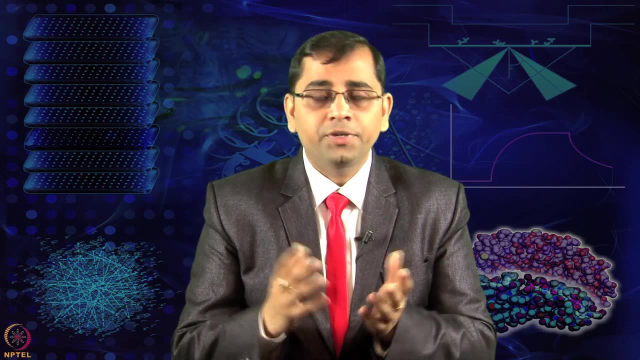 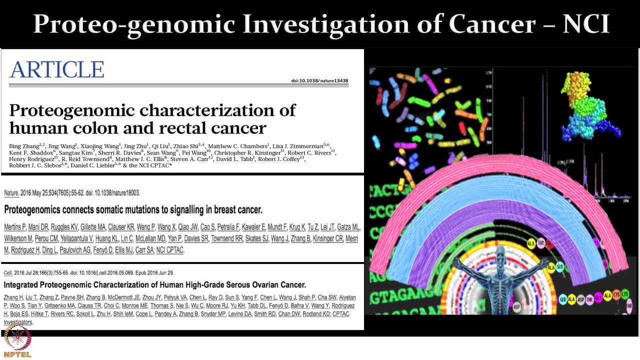 functional consequence of somatic mutations, narrow the candidate nomination for the driver genes which may have the large deletions or amplified regions, and probably identify the therapeutic targets. The National Cancer Institute and National Institute of Health in USA. they have really made huge contribution in this area of proteogenomic investigations. There are series: 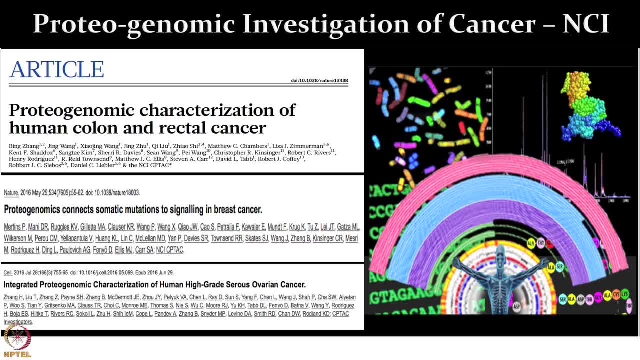 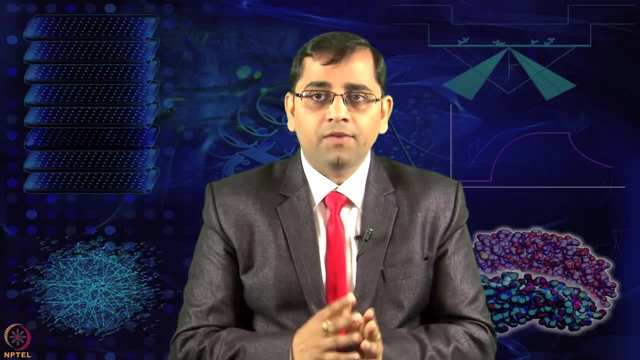 of interesting paper which I have shown on the screen. They have shown the utility of integrating these technologies and how one could actually understand the very complex cancers in much more efficient manner. especially the studies on the colorectal cancer, breast cancer and ovarian cancer have really given. 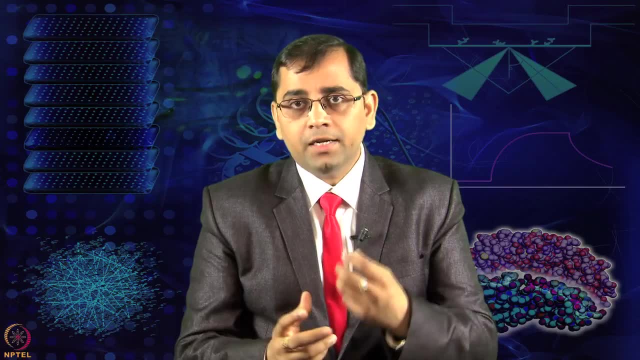 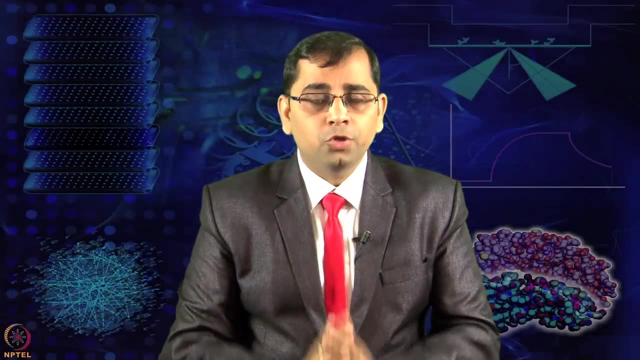 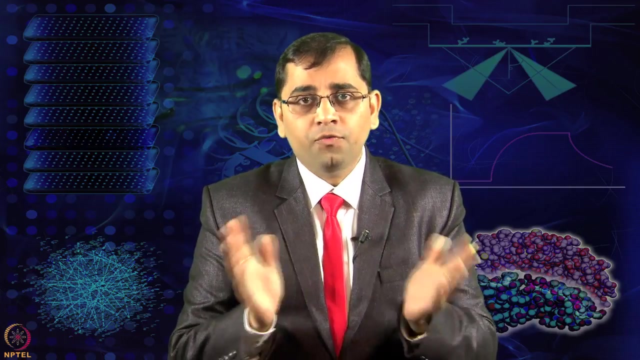 the path that how to integrate this information and get much more meaningful insight for the same complex disease which was otherwise not possible. So in the field of proteogenomics, which actually we offer another course on this, this is a much complex subject and requires much more discussion, but to give you a flavor, it involves: 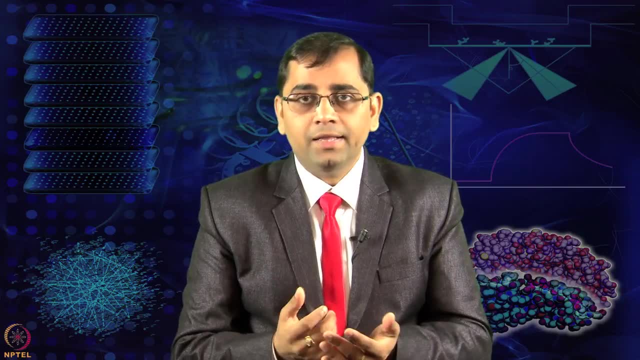 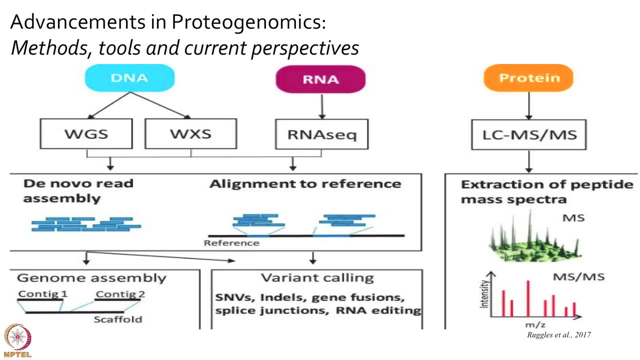 on the same sample and it is more used in the case of cancer and other complex diseases. from the same patient sample can we look at DNA and look at their whole genome sequence and whole exome, Then look at the RNA analysis, RNA sequencing, entire transcriptome analysis and protein and 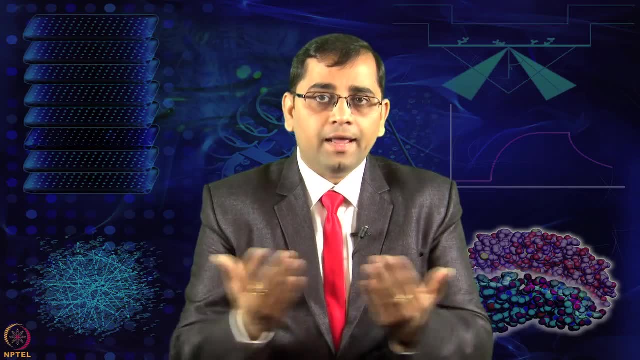 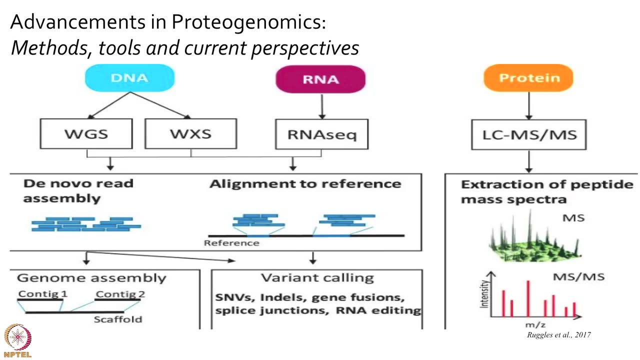 analyze using LC-MS-MS and then start aligning the data, start analyzing the data, big data, to obtain the proteogenomic information which has given those paper which I just showed you in the previous slide. There has been many beautiful studies which have shown the 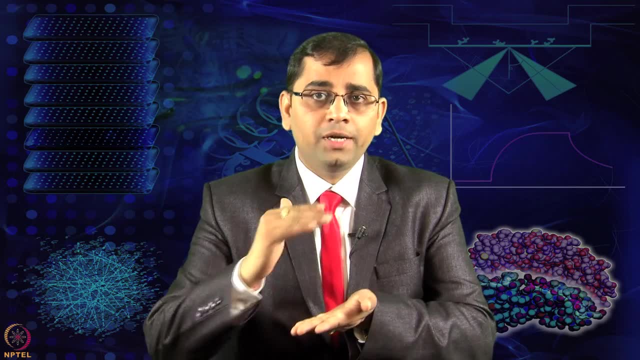 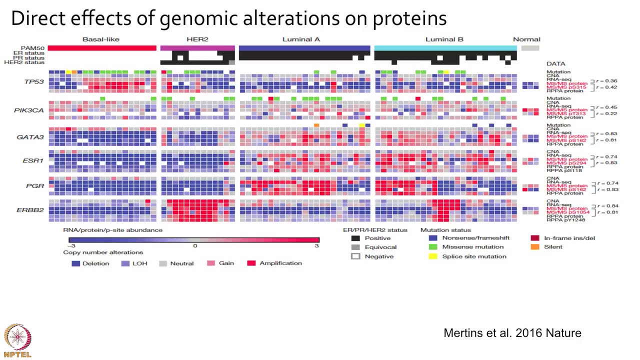 impact of these studies and they have also shown that you know how, if you build the layer wise information, as you can see in one of this nature study shown in the breast cancer, That if you are looking at different subtypes, like basal, like HER2, luminal A, luminal B, these 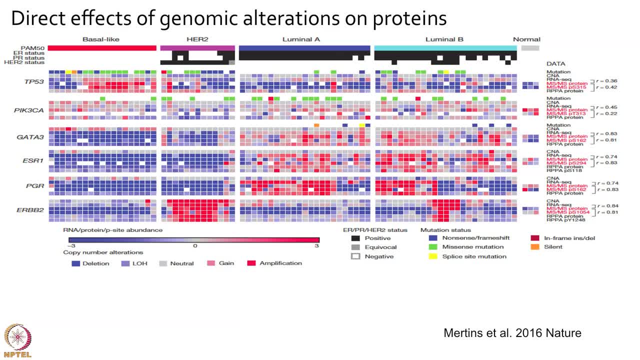 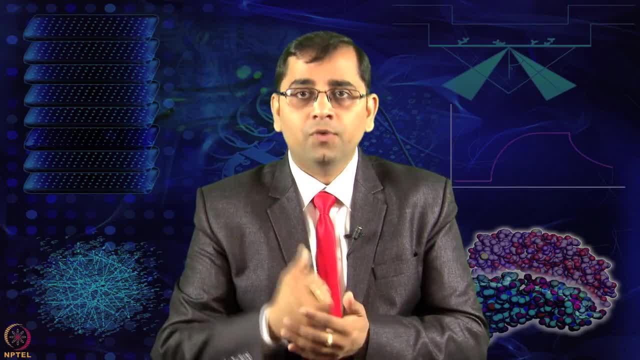 cancer type. if you are only looking at one layer of information, only at the gene level, or even only the protein level, that may not help you to obtain the entire picture, But even sometime. information at the phosphorylation level, or PTM level, is much more powerful than 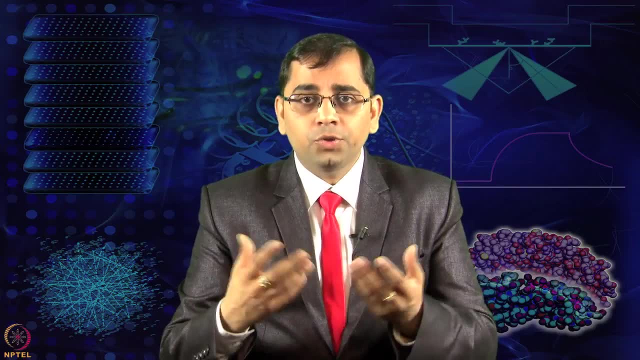 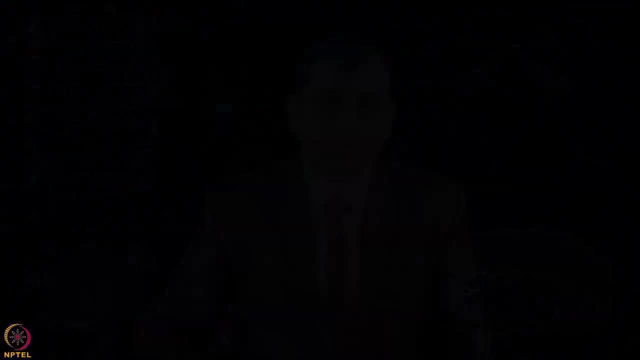 just looking at all of this other molecules. So you have to, you know, get an idea that how this entire information can be put together and can give us much more meaningful insight. So, based on this idea that, how to utilize these omics field, omics technology, the ex 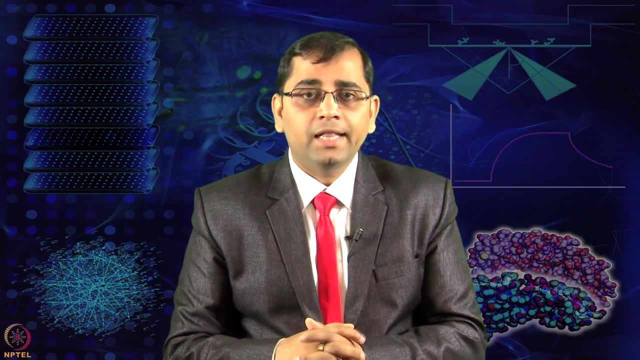 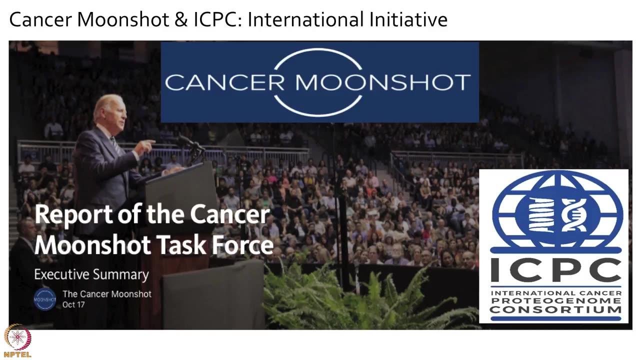 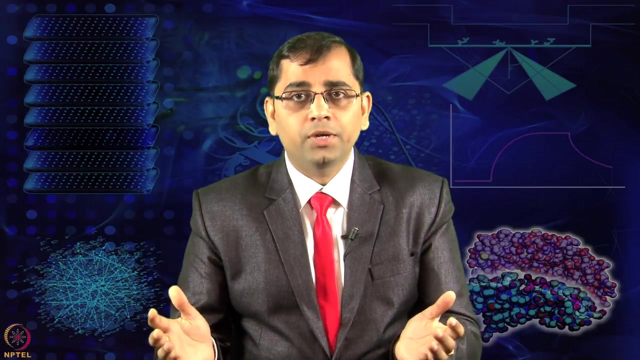 US vice president, Joe Biden. he started the project cancer moonshot Idea was: can we accelerate our pace of doing cancer research and whatever we are able to achieve in next 20 years can be achieved in 5 years. So in this manner, scientists really got motivated and started coming together in the field of. 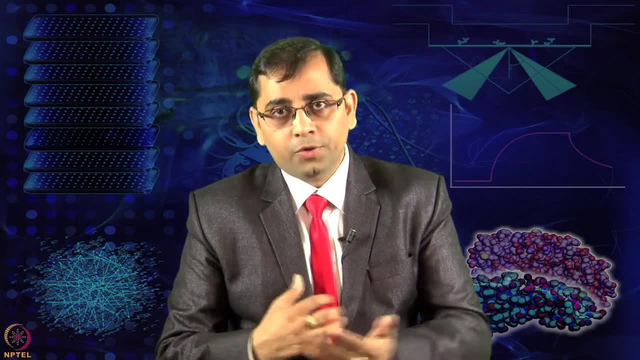 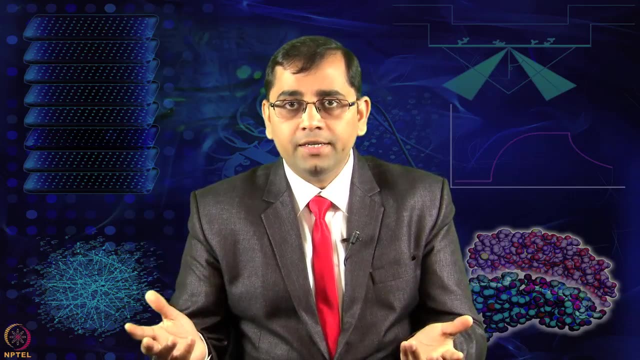 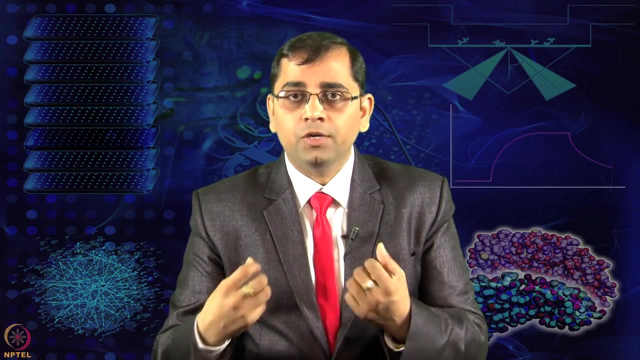 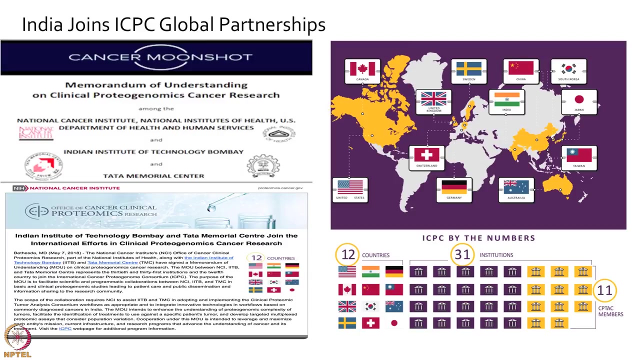 proteogenomics which led to the cancer moonshot USA program. The next intention was: cancer has no boundaries. can we expand this project to the international community? and they form international cancer proteogenome consortium to have more association and collaboration from other countries. We are very fortunate and proud to be part of this program of ICPC, where India joined. 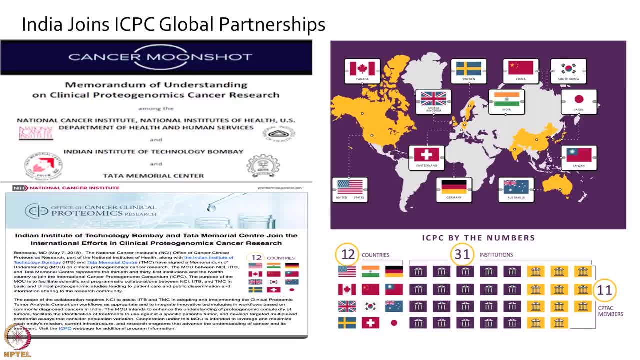 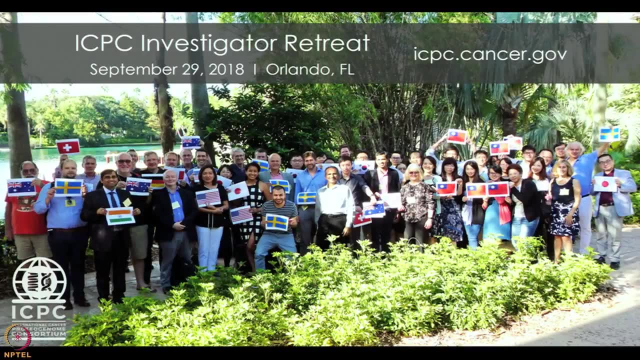 the 12 country consortium and we are also going to look at the proteogenome analysis of different complex cancer of India and then share the data and analyze the data with different countries and try to obtain more meaningful information for these difficult to treat cancers. An image shown here for one of the ICPC retreat where different countries are participating. 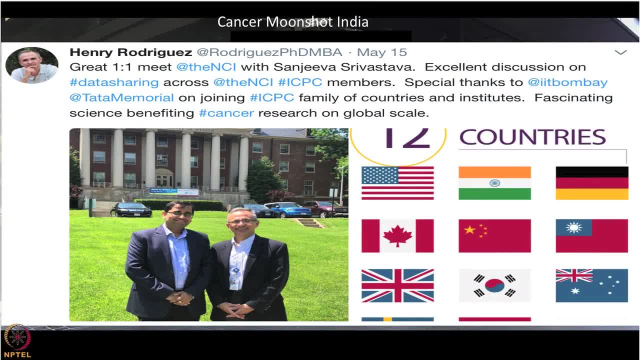 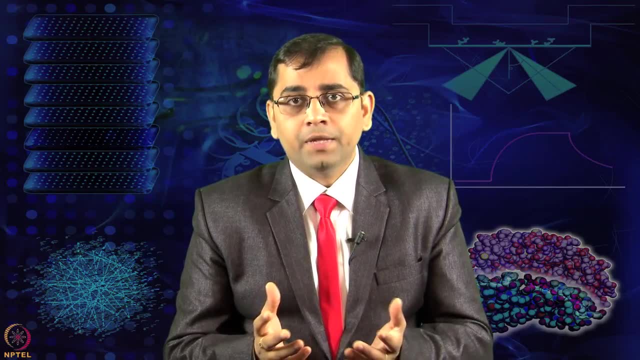 in this activity. So in the picture I have shown Dr Henry Rodriguez. he is one of the director of NIH, NCI who has really led the path for the ICPC program and I am going to show you This is a video clip of sharing his perspective about the ICPC program and cancer moonshot. 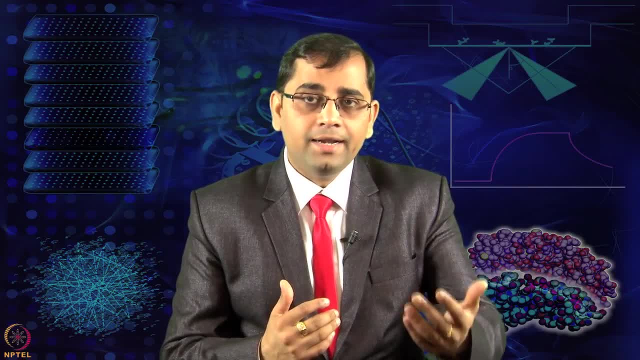 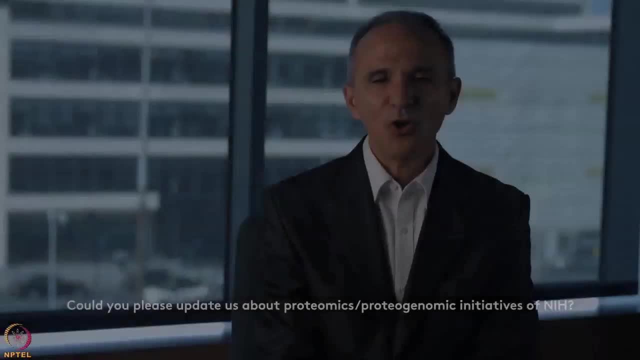 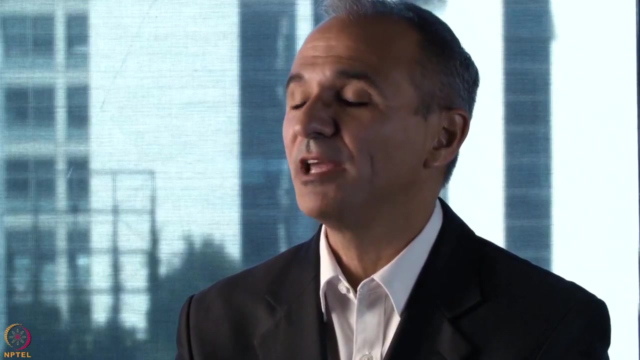 as well as what are the guidelines for doing research in this area and the way forward, his vision. So what I can speak to is the work from the National Cancer Institute, which is the effort that I lead. I think the part that is very exciting is have watched now the evolution, as I would. 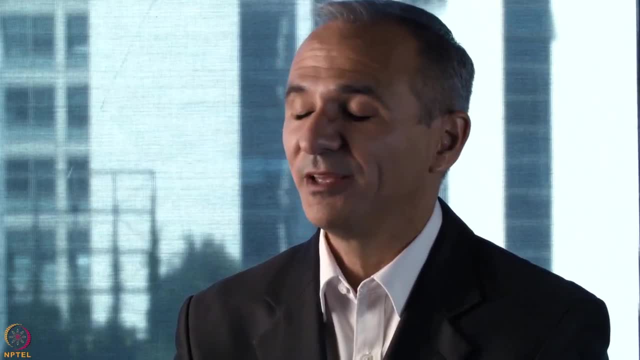 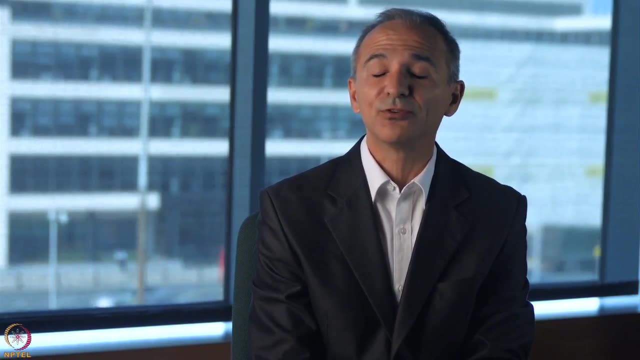 call it, and the maturity of the science of proteomics. So 10 years ago, when we started this program, we were doing a lot of research. We started this effort at the Cancer Institute referred to as now the Clinical Proteomic Tumor Analysis Consortium, CPTAC. there was an acknowledgment out of NCI while we saw 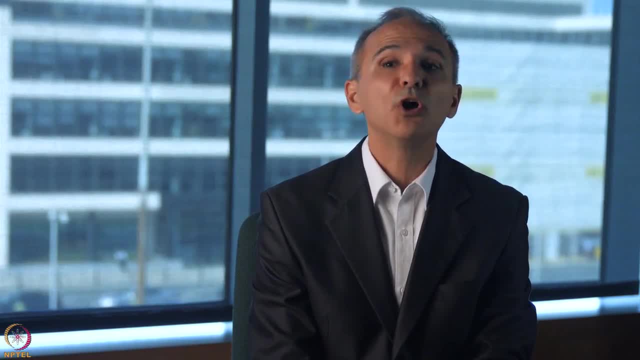 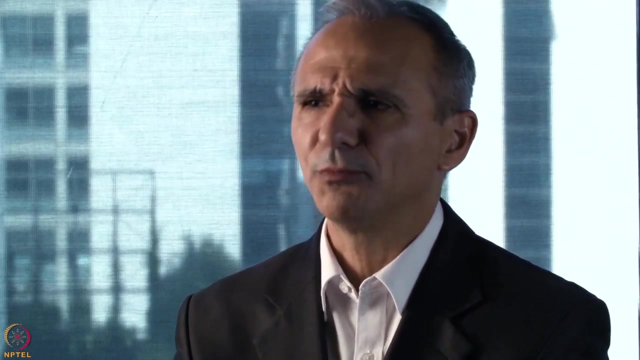 the potential for genomics. We knew proteomics would be a very complimentary field, but at that time we felt the technology that was being developed, in this case, mass spectrometry. yet, while it is extremely, a very powerful technique, there were items that we needed to address in terms of the rigor. 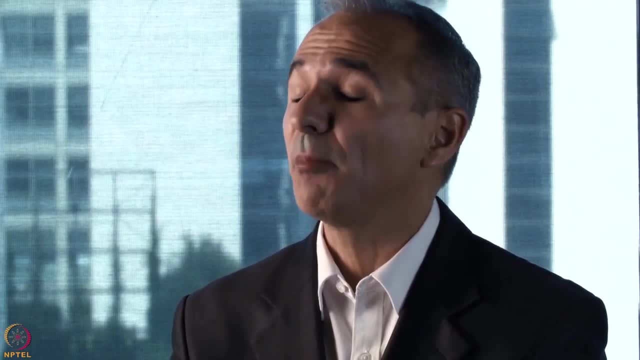 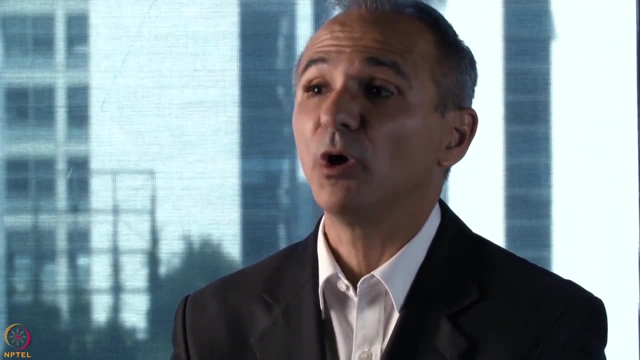 and reproducibility If it were to one day be a complimentary technology to the genomics landscape. So 10 years ago, while the Cancer Genome Atlas was the very first one large scale biology that we moved forward in cataloging all the perturbations inside cancerous cells from, 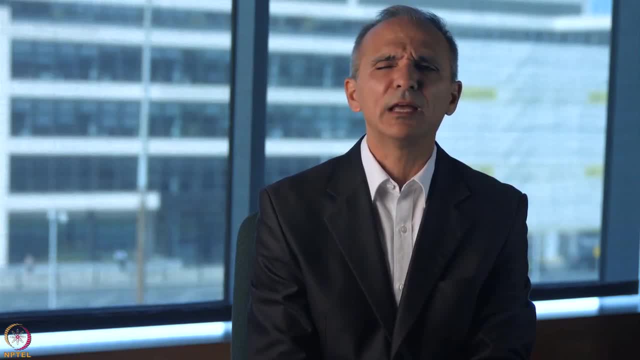 a genomic perspective, the proteomics field. we decided to take a little different approach. We went after the analytical rigor of those technologies. It took about five years. but once we got that finally on hand, the question became: what would we do next? There was the opportunity that we seized. 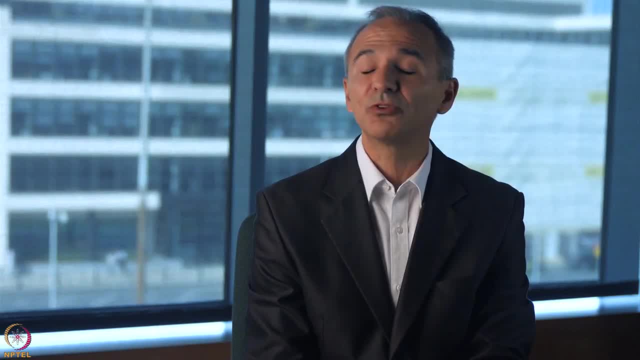 We went after those same tumor types that the genomics community went after in TCGA and we applied those proteomic based technologies- mass spectrometry- onto them. When we saw the beauty of the additional biology of starting to be generated from the combination of these two disciplines, that's when we saw a lot more potential. 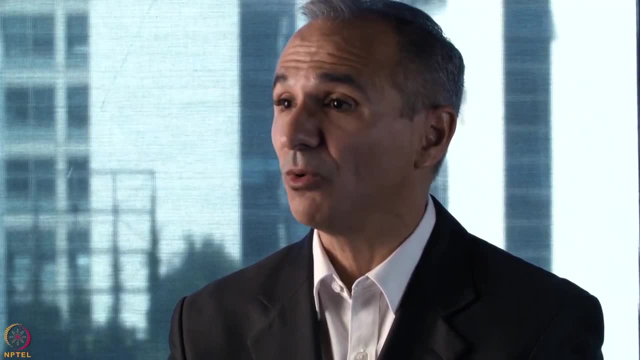 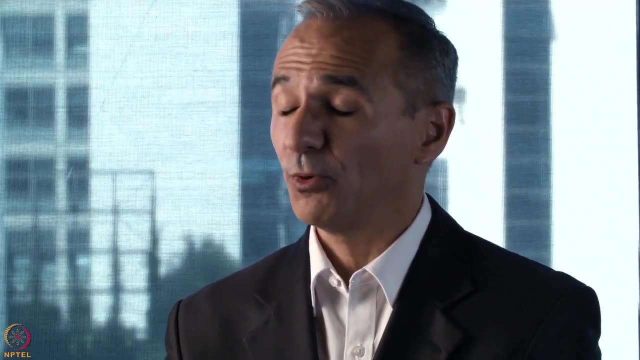 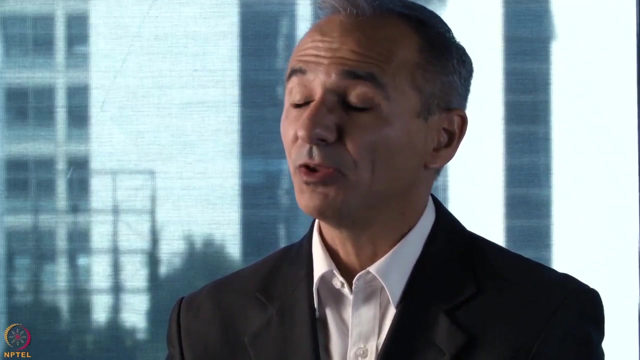 So today this program, now in its next iteration, The way it is, it will be expanding. we will go after additional cancer types from the first program. so the first program we went after colorectal breast ovarian cancer. now we will be cataloging approximately additional five cancer types. but the most exciting part that i would have to say for the first time, 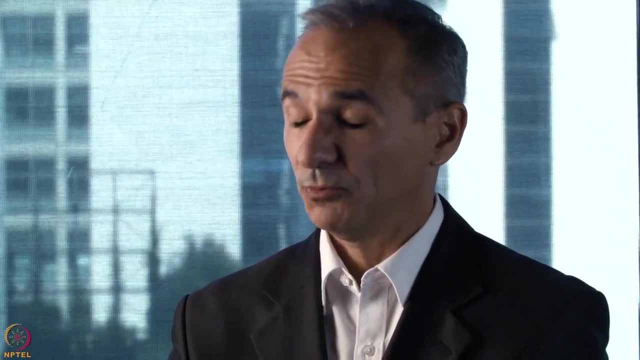 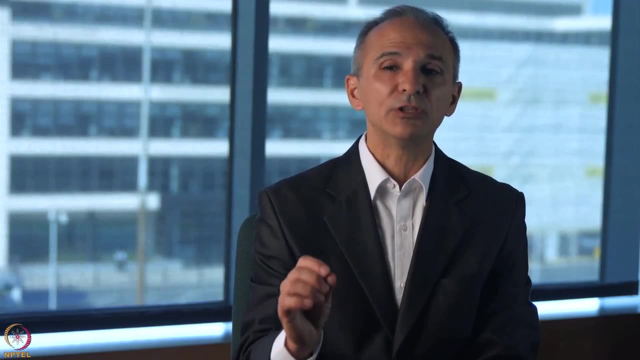 we're going to be teaming up a proteomics laboratory expertise with an ongoing nci sponsored clinical trial, and these clinical trials are typically genomically driven. but we recognize that genomics is still advanced. but there's an opportunity to fill in the void of the biology, of trying to understand why patients either respond well or do not respond. 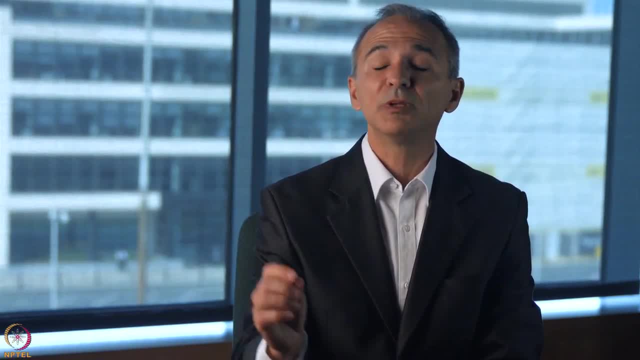 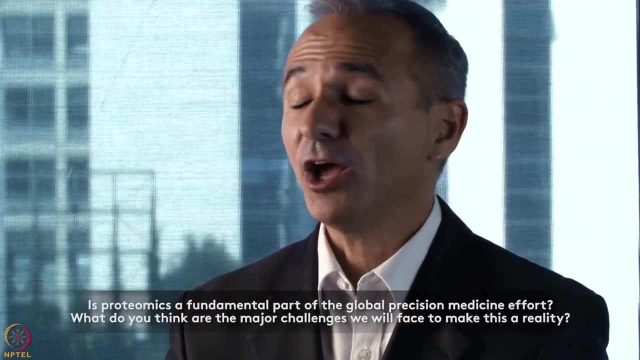 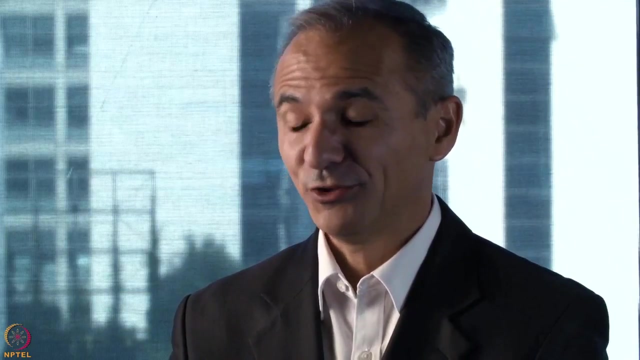 well, based on a genomic driven information, to the treatment that they were just administered to. i'd say the best way that i would look at it is what is driving precision medicine today? in oncology, which is my specialty, i think clearly genomics is making tremendous strides. they're 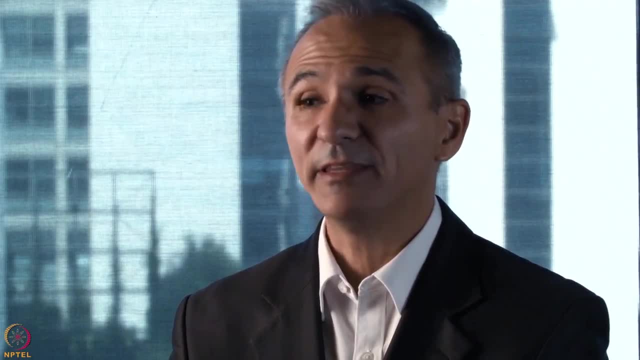 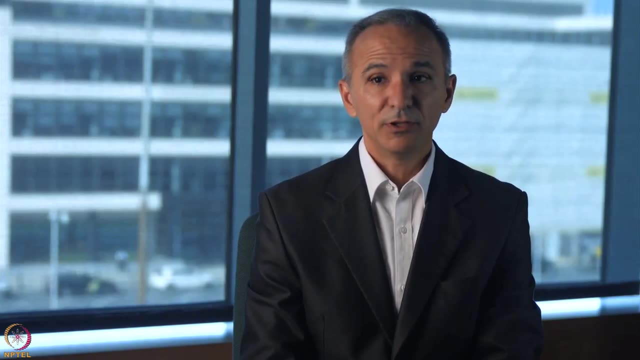 again exquisite examples today where we're able to identify and be in a very great position on how to treat a patient, simply relying on genomics. however, you gotta flip your coin. there are still many instances in oncology where you do not fully understand the biology and how these individuals 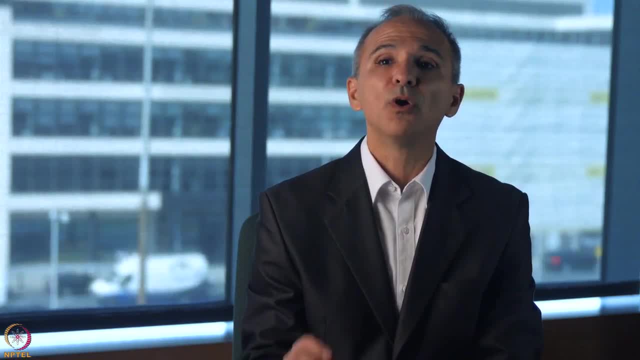 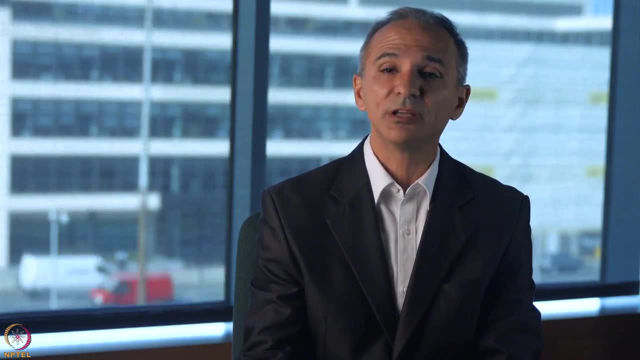 are responding to their treatments. that's where i see now proteomics filling a very critical piece of that information. so what we're trying to do at the nci, through our initiatives, is to begin to converge these disciplines and, quite frankly, partly i think the reason has been is: 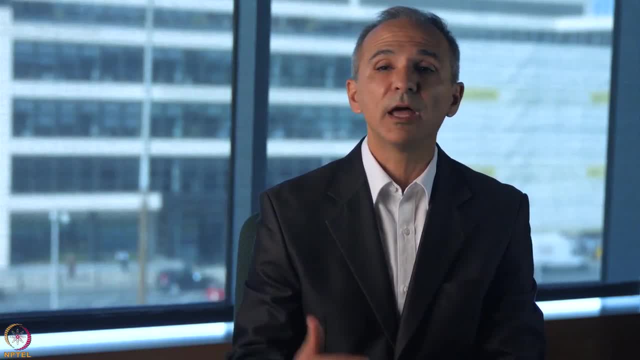 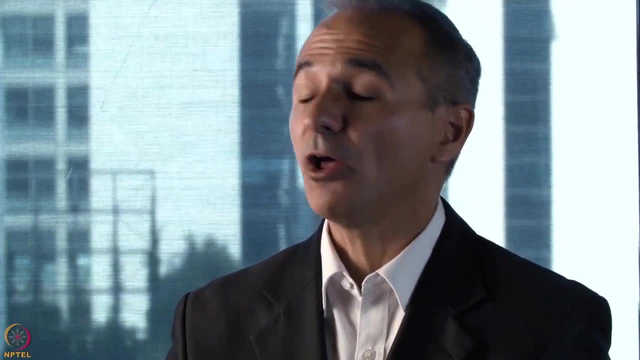 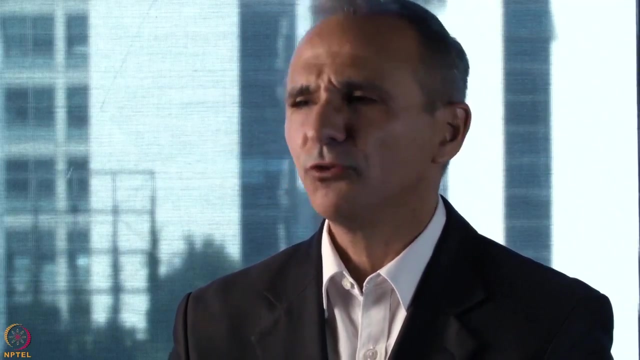 the evolution of technology. genomics technology has matured and is still maturing at a faster rate, but as proteomics technologies are also maturing and also we could go after smaller samples, it's just a matter of time that these disciplines do begin to converge. so that's where i see these. 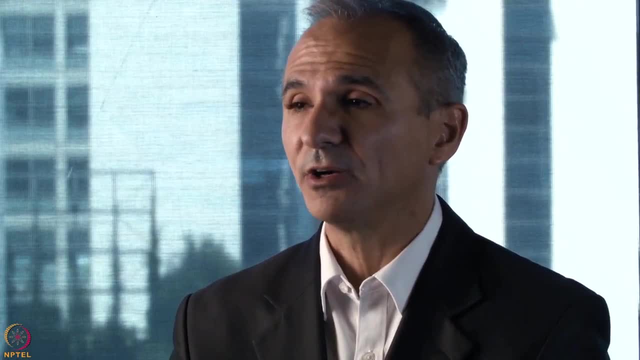 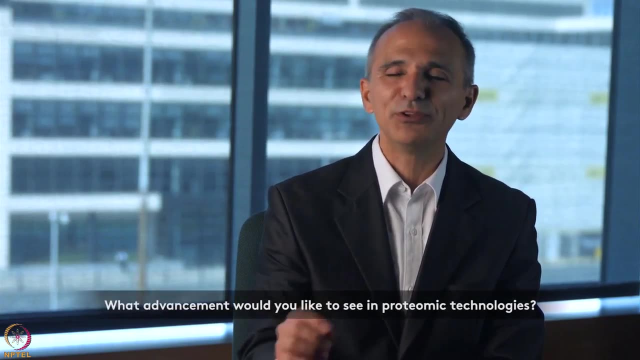 two areas being very complementary to one another. specifically in the area of precision-based medicine for oncology, as opposed to the common problem of mass spec, i would say what's needed, because i really don't see them as problems, i just see them as the evolution of technology. my one wish, i think, 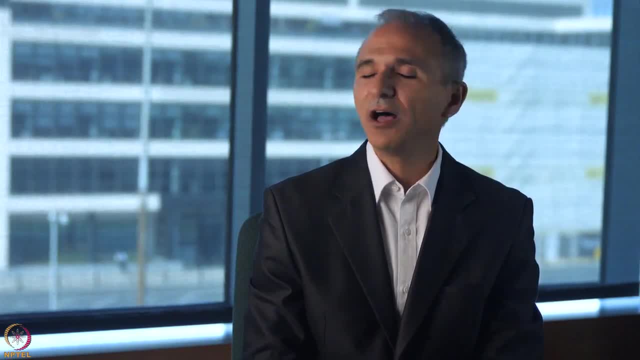 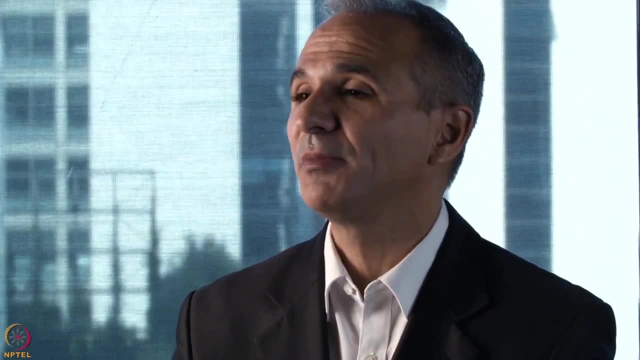 which is a natural wish that you have. of all technologies, the common ones- you want automation. you want it to be very simplistic for the average user to use. you also want that the system, as technologies evolve, to potentially be using less sample material up front. but keep in mind, i think, 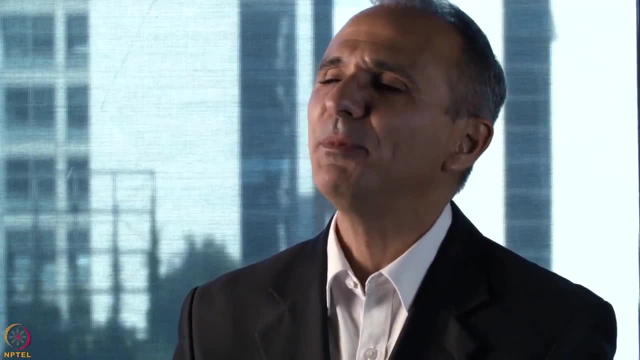 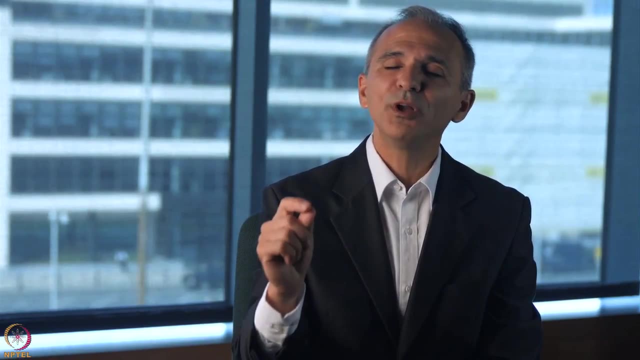 this question is one that people tend to ask me a lot, and i think it's one that people tend to ask on is: well, how much material do you need to do? the analysis that you wish to go after the question that people should be asking is: what do you? what is the question you're trying to ask? 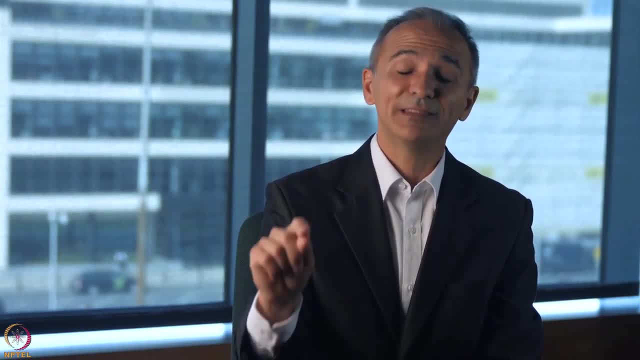 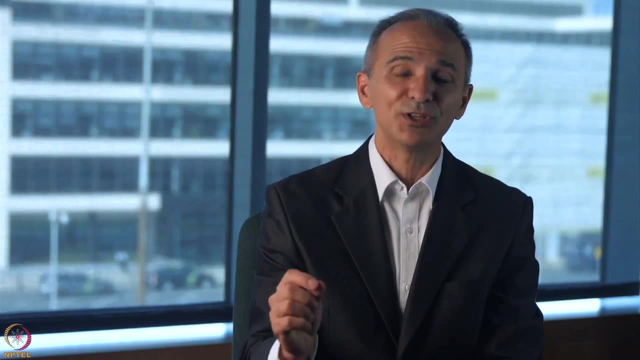 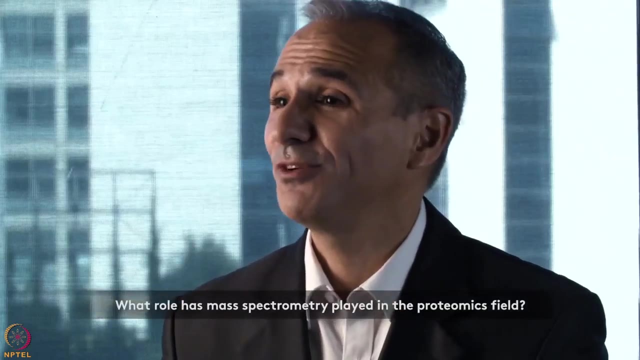 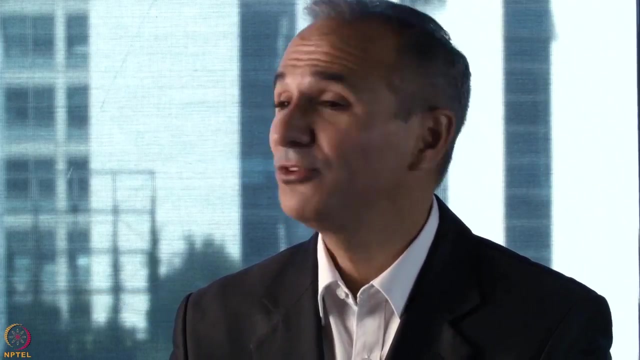 of the biology. that question will dictate what you want the technology to do, and in most instances you find out when people really begin to ask the question they would like to see of the experiment. technologies themselves are quite mature. from what i've seen from my perspective, you know what i think about the genomics the way we know it today would not exist without mass. 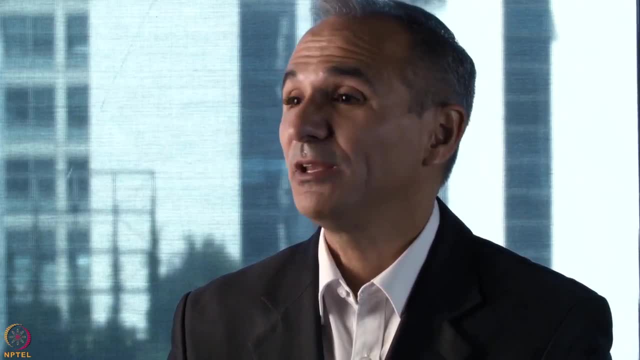 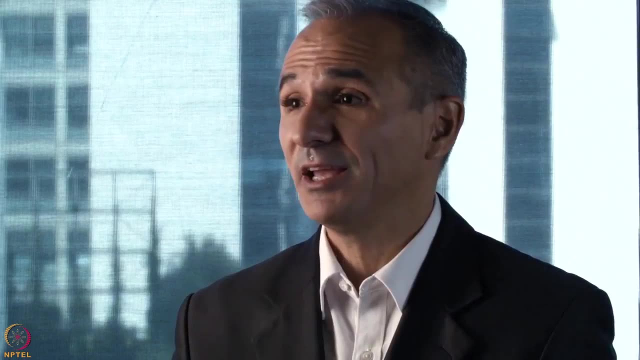 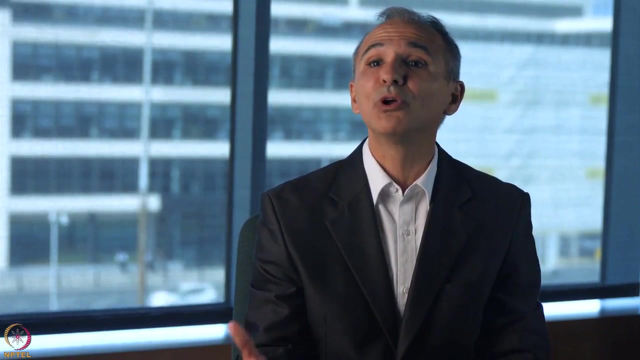 spectrometry. pure and simple genomics gave us a blueprint what people did within the specialty is. there was an acknowledgement. here is a mass spectrometer. mass spectrometry has been used in clinics for over 30 years for different purposes. it's mainly used for small molecule screening. 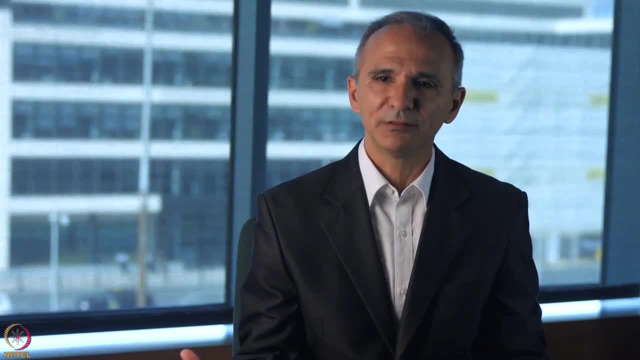 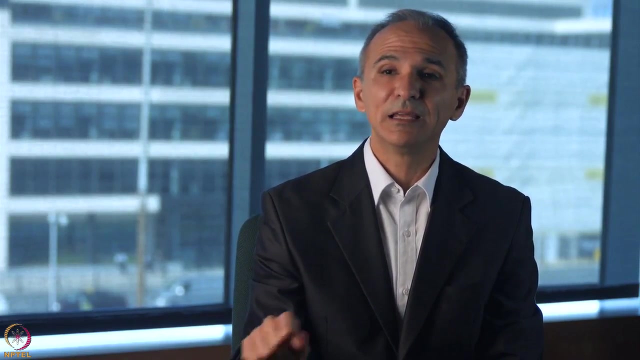 but then a bit. but then there was a brilliant idea that came into play: can you take a big protein, break it apart into small pieces, into these peptides and informatically, just like an eloquent puzzle, stitch it back up into a protein? without mass spectrometry, proteomics as we know it today simply would not exist. so the cancer moonshot. 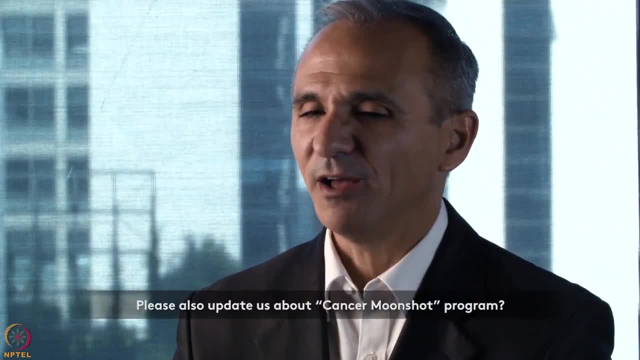 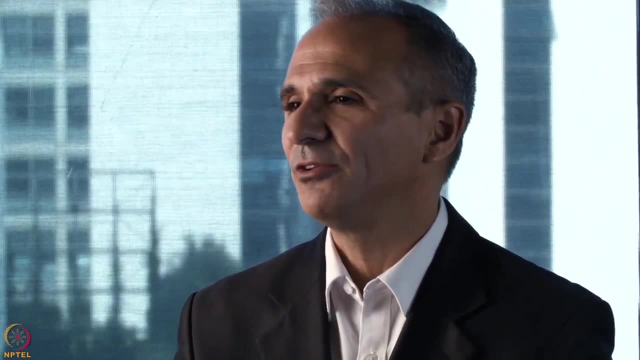 i'd say is one of the most incredible things that's been developed off the united states over the past. uh, now what? approximately one year. so obviously one of the main drivers here is is is the 47th vice president of the united states, joe biden. it's been a huge honor to be. 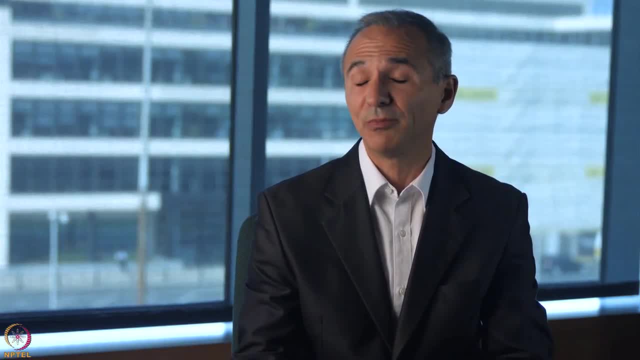 part of that effort. he's been the first in the country to have a program called the cancer moonshot umbrella and we've been pushing that forward for 50 years. and we've been the first in the country to have two programs that i could specifically speak to myself on. one of them we actually did, which is 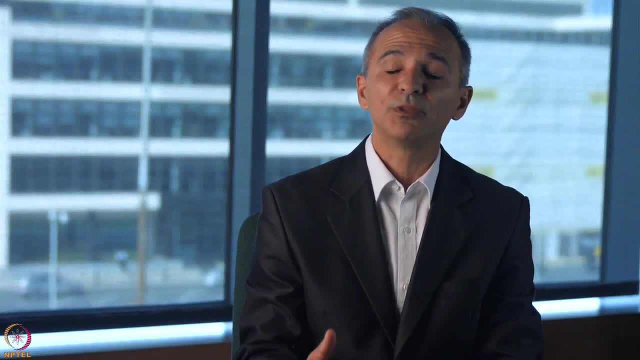 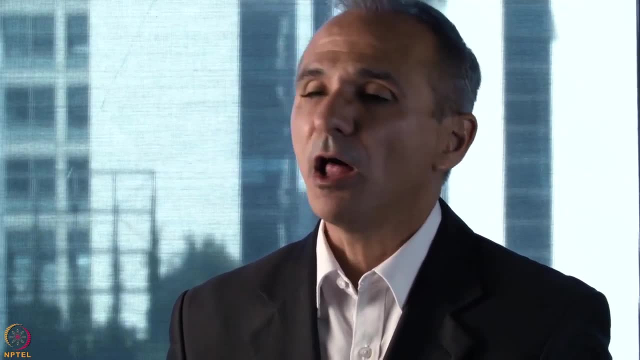 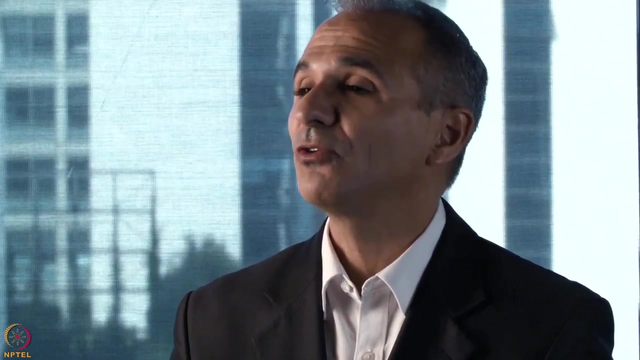 a partnership between the national institutes of health, specifically nci. then we partnered with the department of defense. we also partnered and we also partnered with the veterans administration. this program is referred to now as apollo. this effort, along with another program that we've now now, is referred to as the International Cancer Proteal Genome Consortium, or ICPC. 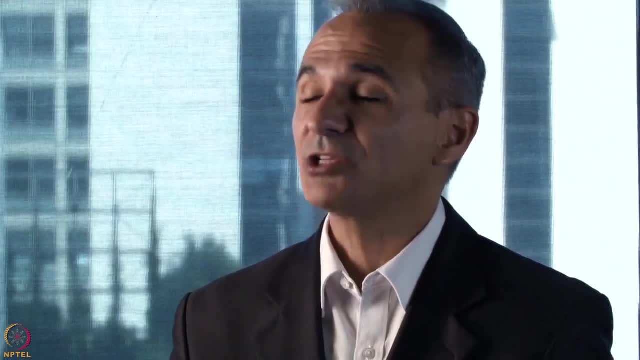 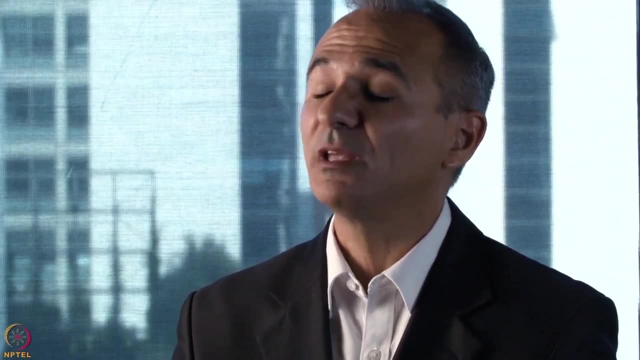 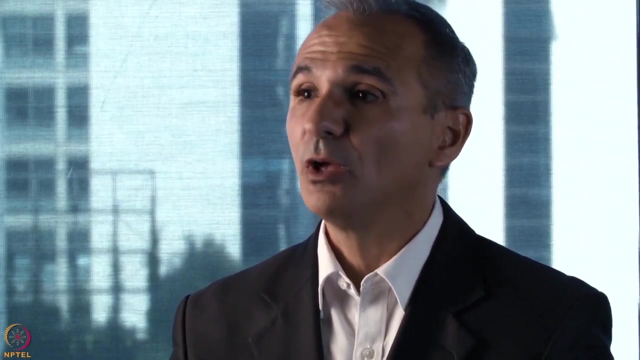 That program now, which is an incredible effort in itself, actually now involves 27 institutes, spans 11 countries. What's nice about it? it fills one of the key promises that our former vice president wanted, and that is the data that we generate in this international effort will be placed. 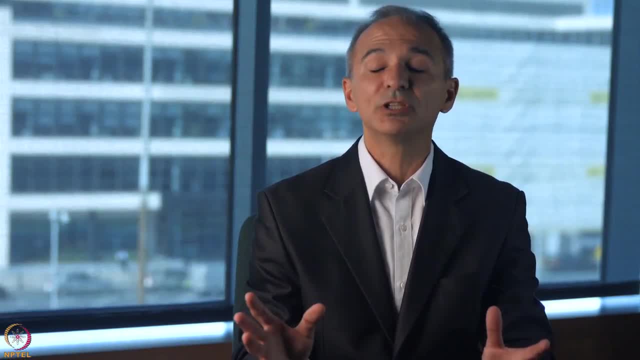 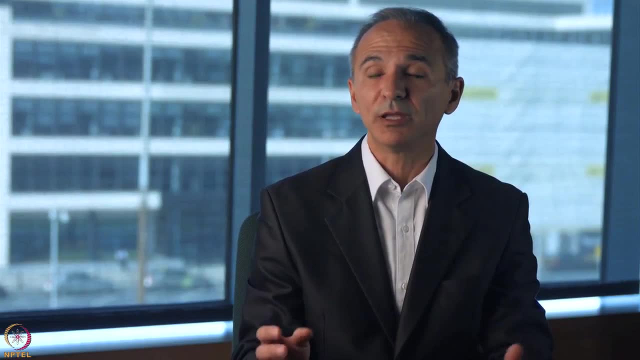 in the public domain. But the part that's nice about these two initiatives is that each one of them ICPC and also the Apollo that will also be giving up the data in the public. But what brings them together? it is the foundation of what CPTAC actually did. 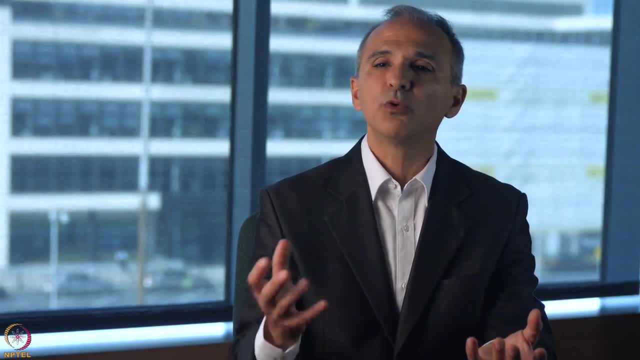 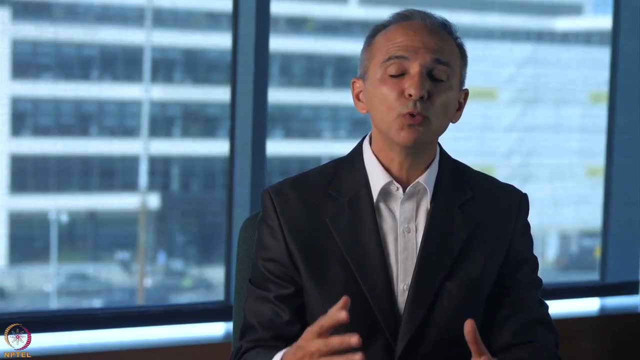 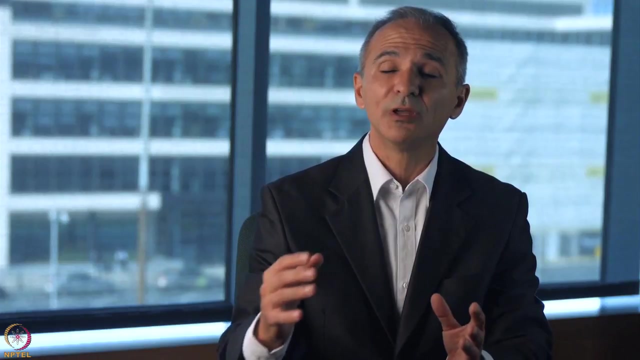 And that is a recognition- converged genomics with proteomics, with the hope that not only you will identify a new biology, but, as in the Apollo case, they really want to push it much more faster in the translational space And potentially, in the near-term future, begin to apply it towards patient care. 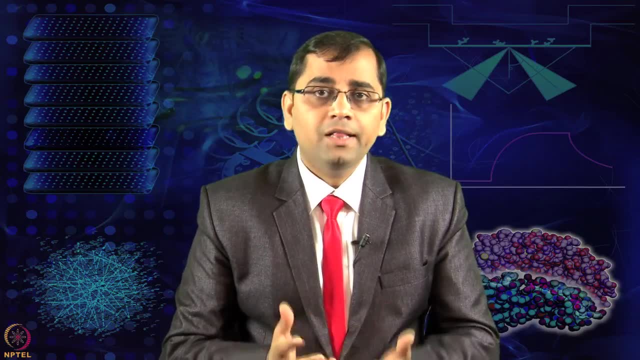 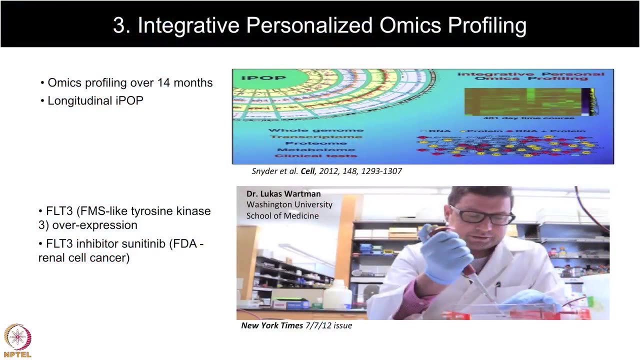 Another interesting development happening in the field is integrative personalized omics profiling. Essentially, this path was led by Dr Mike Schneider from Stanford University, who took his own samples and analyzed longitudinal manner using various multi-omic technologies, which really led first time idea that he might be prone for diabetes, which was detected. 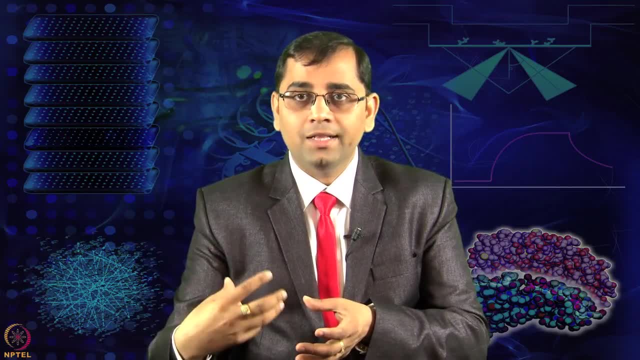 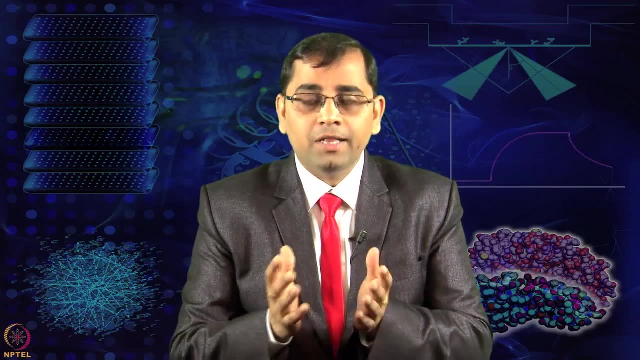 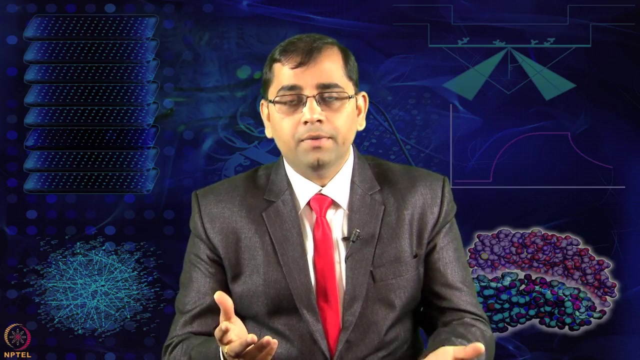 clinically very late, But looking at the biomolecule, they could sense this much ahead of time. And this really constitutes that how, looking at the multi-omic analysis from the same individual can provide more meaningful information. And likewise there are many success stories. many different case studies are now coming. 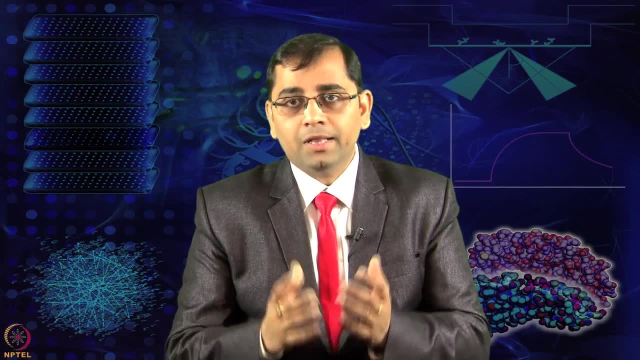 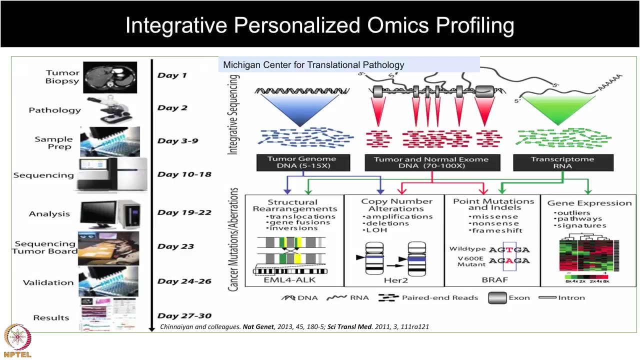 forward which are showing the utility of looking at personalized omics profiling. There are also groups in Michigan who are looking at Michigan Center for Translational Pathology: Dr Arul Chenayan and team. They are doing from the same patient, looking at the genome data, their proteome data, their 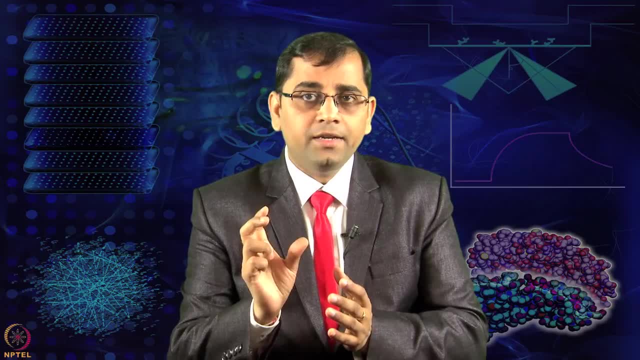 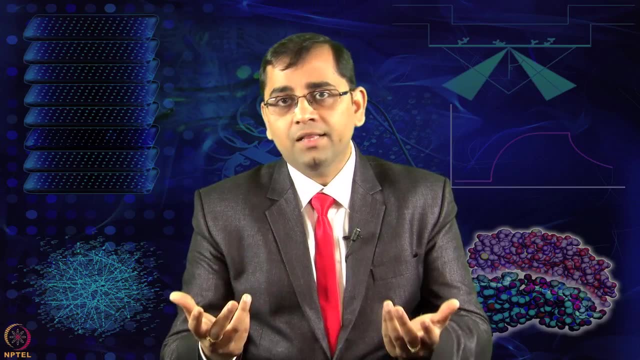 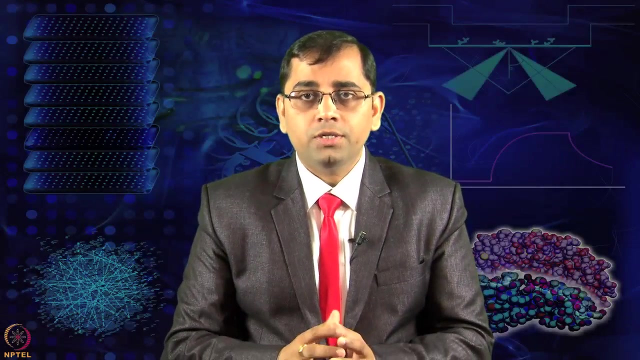 metabolome data how one could start finding the right cure for the given tumor type, which is otherwise not possible, And they are able to provide, at a much comprehensive level, this kind of analysis and directly reaching to the patient care. Now Dr Mike Schneider and his team has launched a major program on human personal omics profiling. 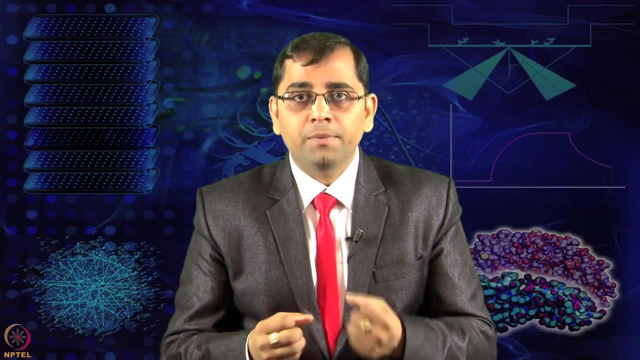 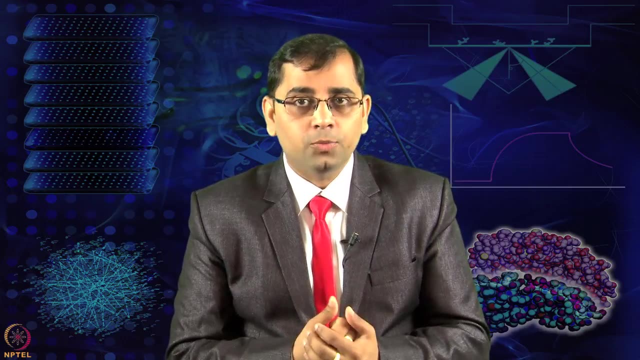 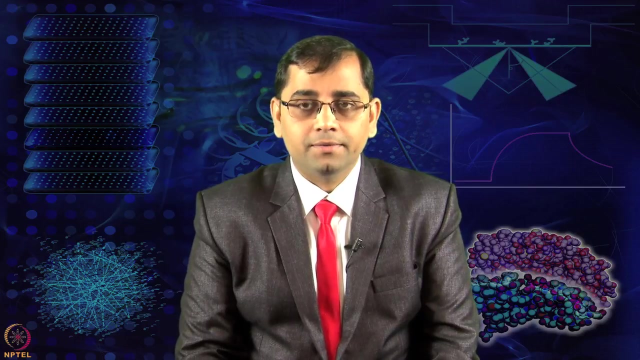 or HPOP, And idea is to provide much deeper understanding, Thank you. And the aim is to bring to the table an understanding of the genetics of the human body and provide the new clues of different diseases which were otherwise not possible. Let's hear Dr Mike Schneider about his program and vision for the HPOP project. 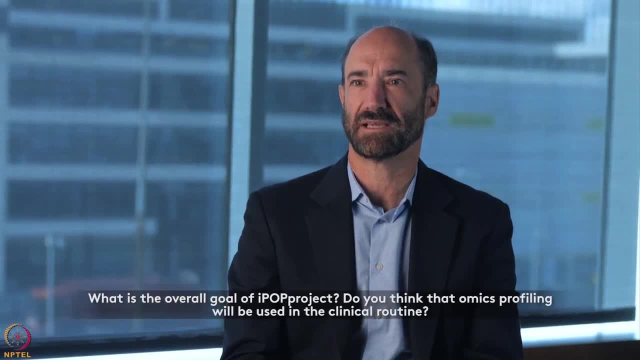 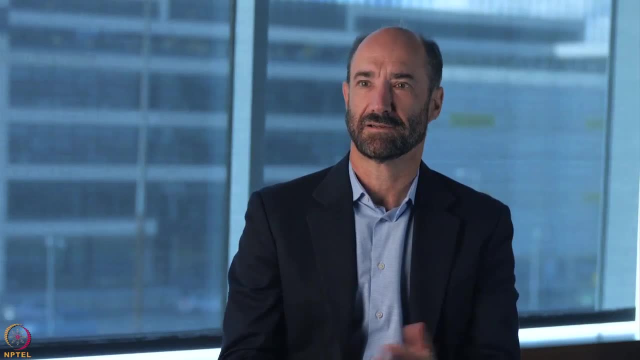 What is the role of the HPOP project? The HPOP project is really trying to understand what it means to be healthy, and how do people differ all around the planet? So what we're doing is we're actually taking people's blood and urine. 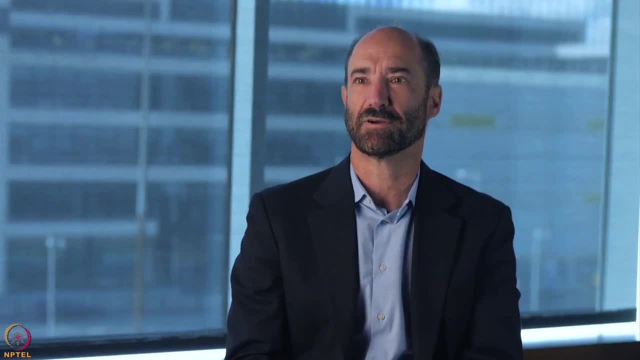 And what we're doing is doing deep omics, profiling the proteome, the metabolome, the transcriptome, to make as many measurements as possible, to see at a molecular detail how people differ from one another. So we're going to see this, we're going to sample people from all around the globe at 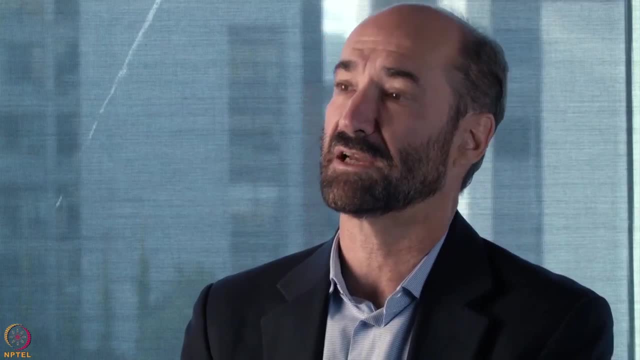 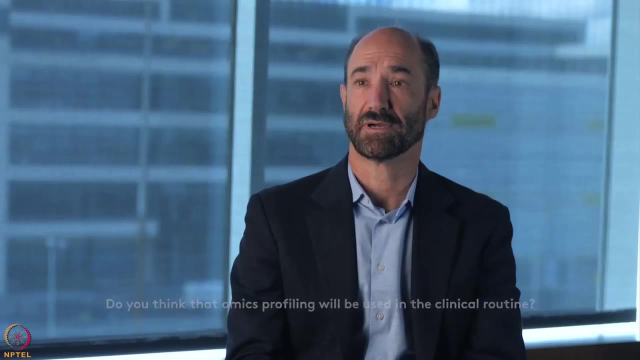 these human proteome meetings and then we're going to see what their molecular diversity looks like. how do different ethnic groups and different locations have an impact on people's molecular composition? Do I think omics will be used in clinical situations? I think at some level, absolutely. 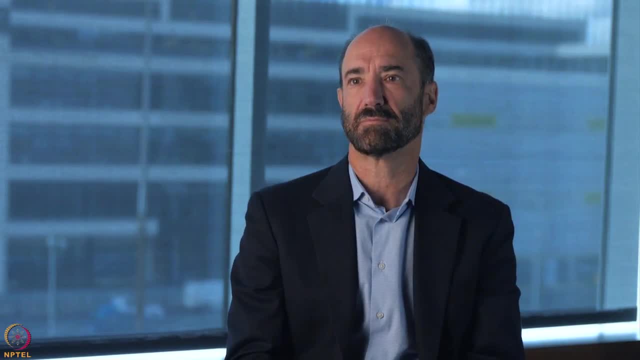 That is to say, we'll be making thousands, if not more, measurements in the future. Right now, when you go to a doctor, they make about 15 measurements on you, and in the future I think we'll be making hundreds, if not thousands, using various omics methods, especially proteomics. 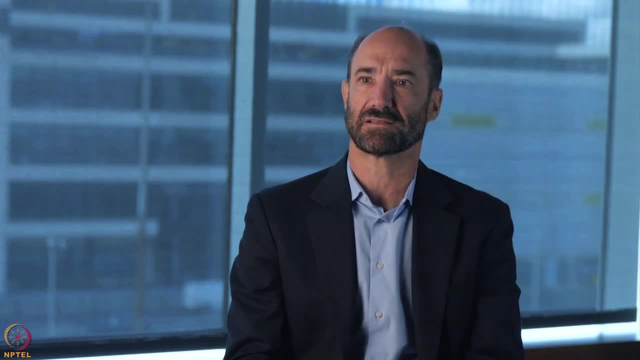 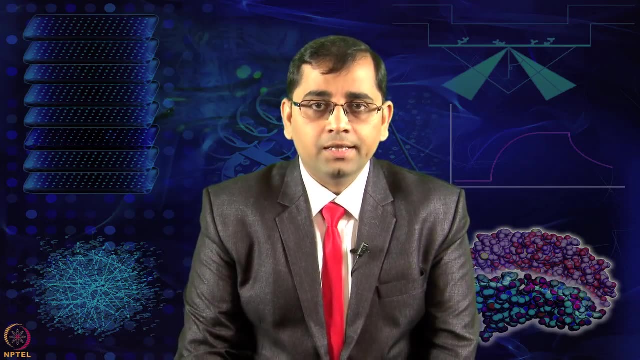 and metabolomics will be very, very powerful for looking at people's molecular state, which I think will say a lot about their health and also what happens when they get sick. Let me now take you to the lab. Let's go to the next project, which is wellness project. 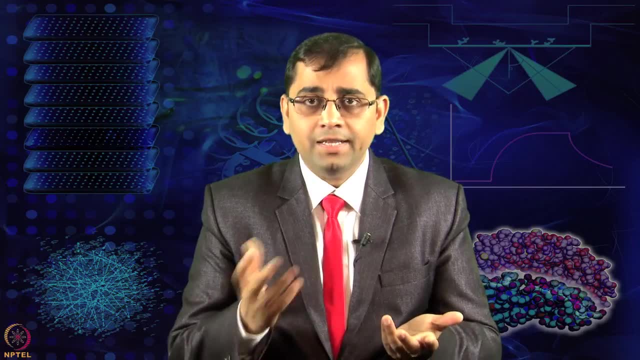 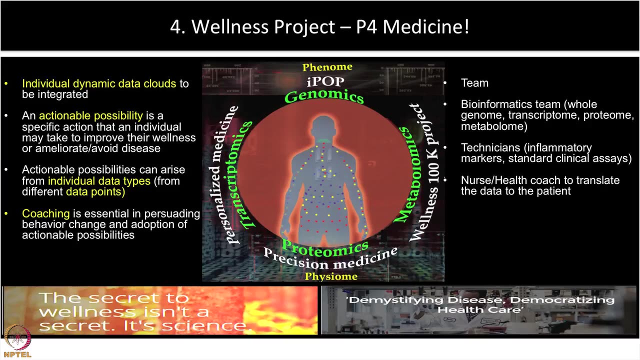 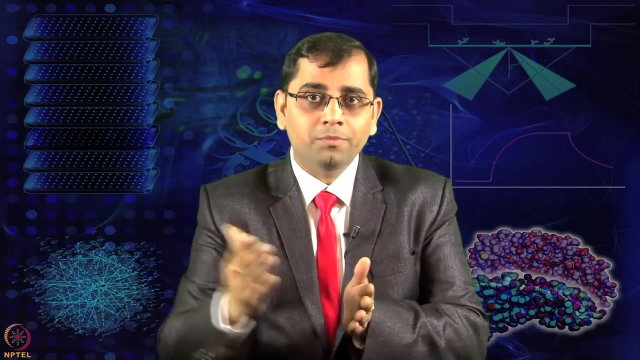 We have been talking mainly about how to compare the healthy individuals with disease. But can we look at the wellness or the health status of healthy individual, or seemingly healthy individual, in the longitudinal manner? So can we look at their entire omics profile at different time interval from zero time? 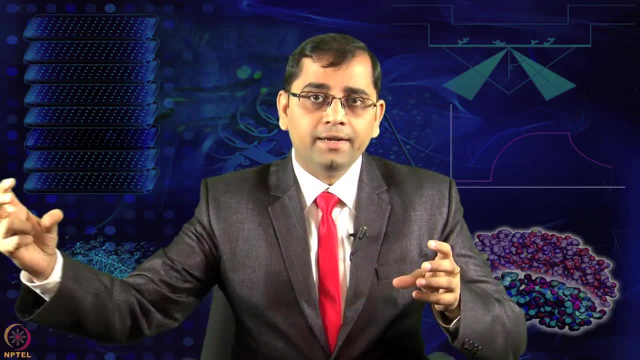 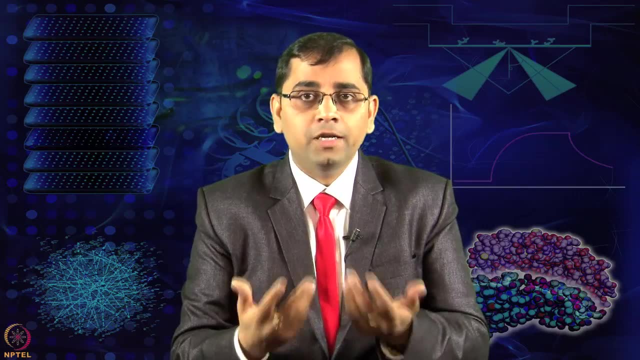 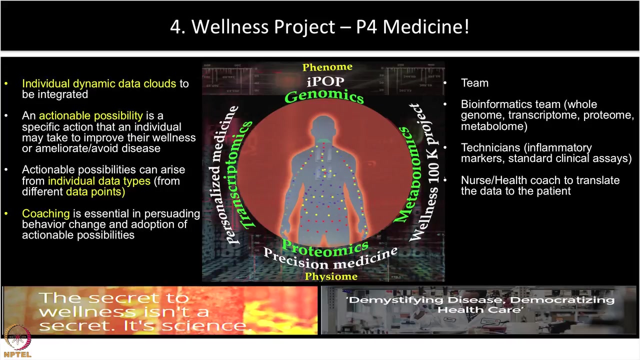 to six months to one year, two years, and start looking at: are there changes happening in dynamic manner inside the body Which might give us the clues For what disease the individual might be having or whether the individual is still healthy? So the individual dynamic data clouds has to be integrated and that field is known. 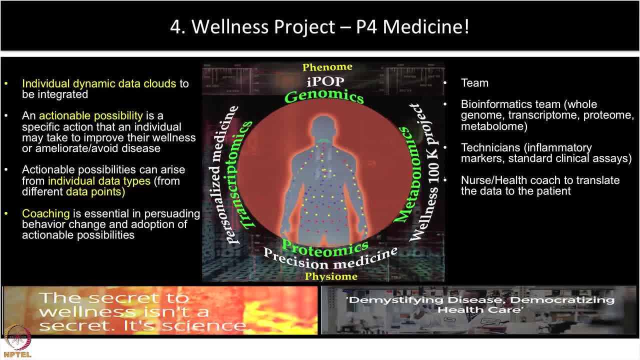 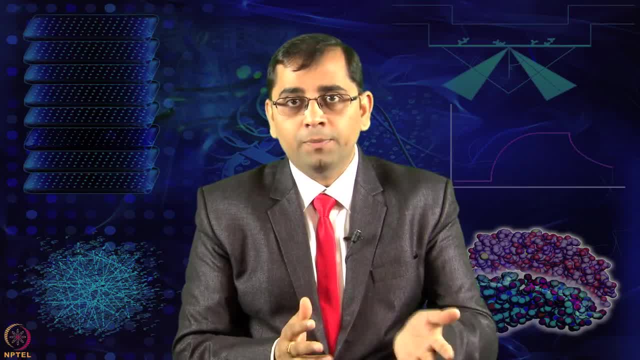 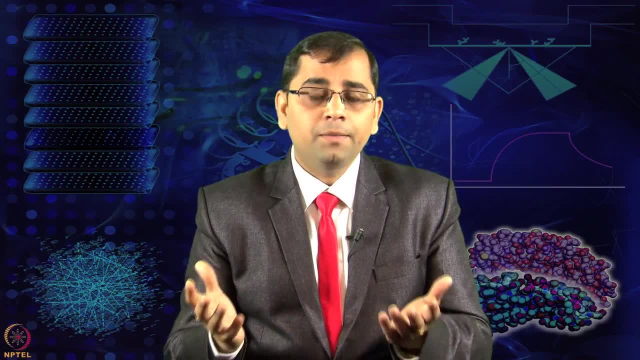 as P4 medicine, which is led by Dr Leroy Hood from Institute for System Biology in US in Seattle. This big project of wellness was also published two years ago in Nature. Biotechnology has shown the utility And many similar projects have now started. 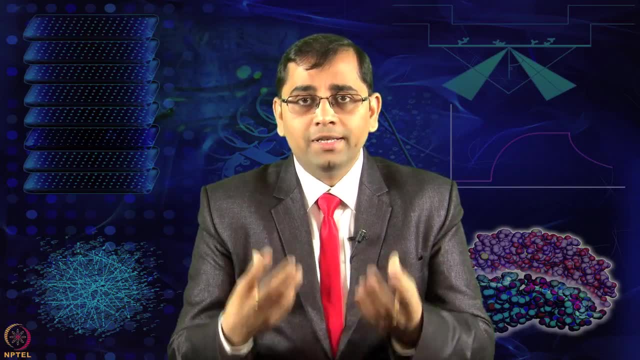 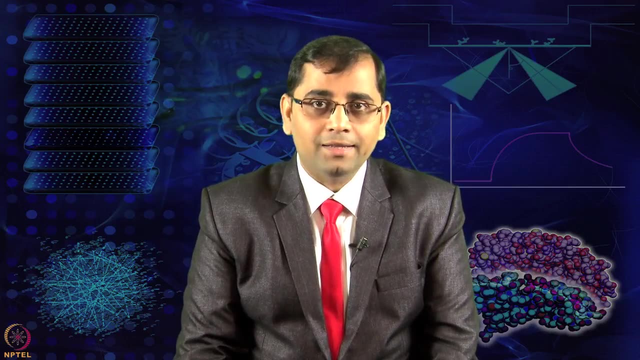 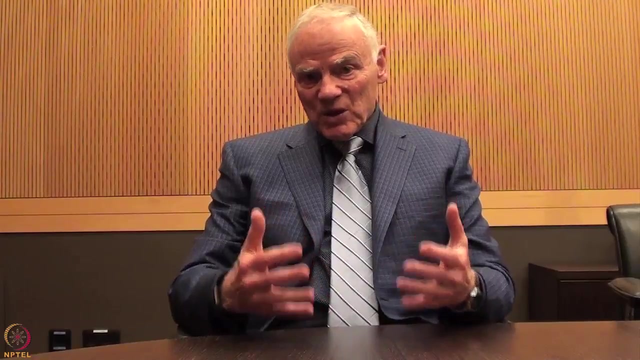 Right In different countries which are looking at the omics data set to build the wellness. Let's hear the views of Dr Leroy Hood on the wellness project and P4 medicine. I'm very excited by the possibility India would consider a scientific wellness program. 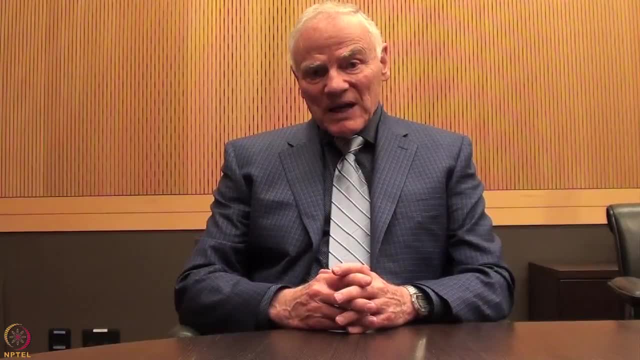 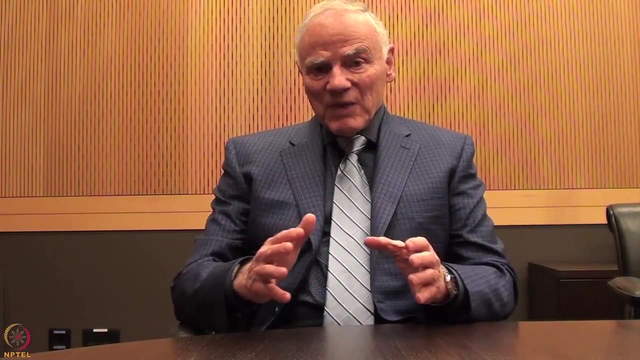 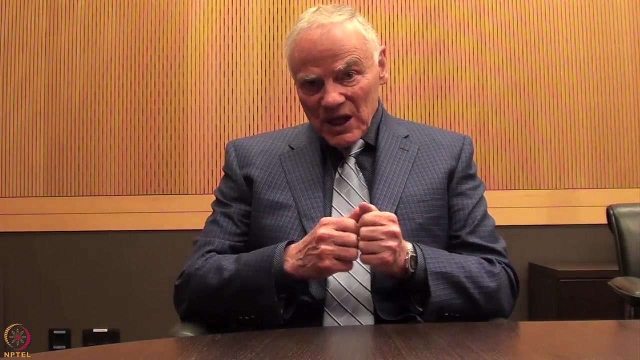 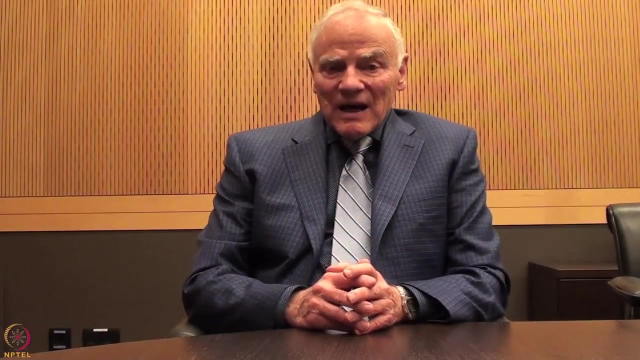 starting with a pilot project in its own population. Yes, Yes, Yes. That's what I think is the keystone for the revolution in medicine, Because, through a longitudinal analysis of populations, using what I term personal, dense dynamic data clouds, that is, the analysis of genomics, of proteomics, of metabolites. 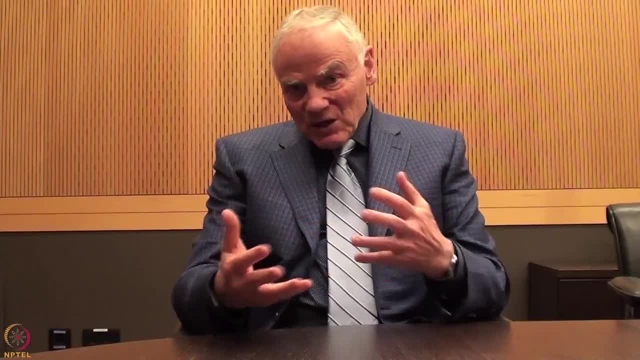 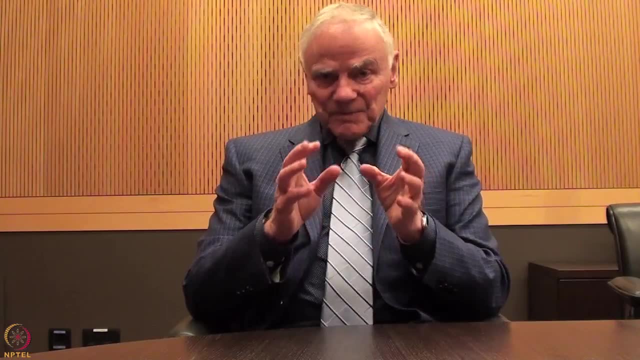 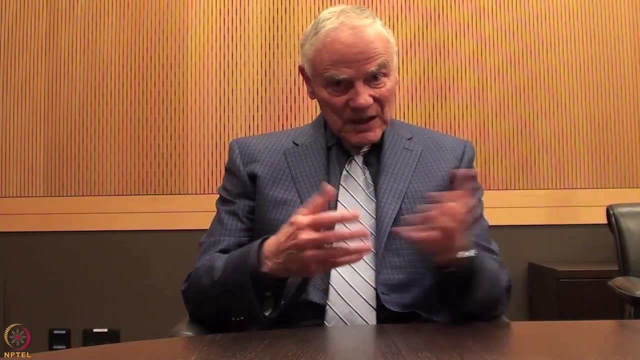 of clinical chemistries, of digital assessments of activity and sleep and things like that. It's one of the most important things, and sleep and things like this- all of these together, when analyzed properly, can lead to actionable possibilities to improve wellness and or to avoid. 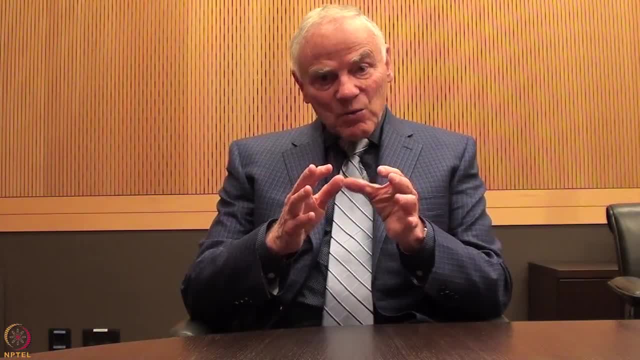 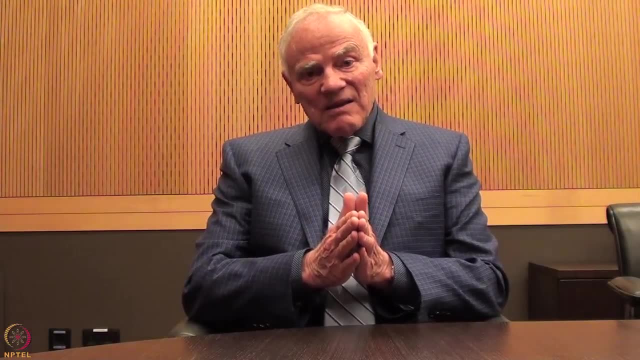 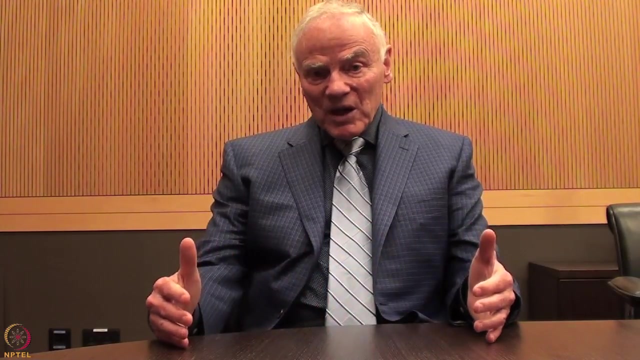 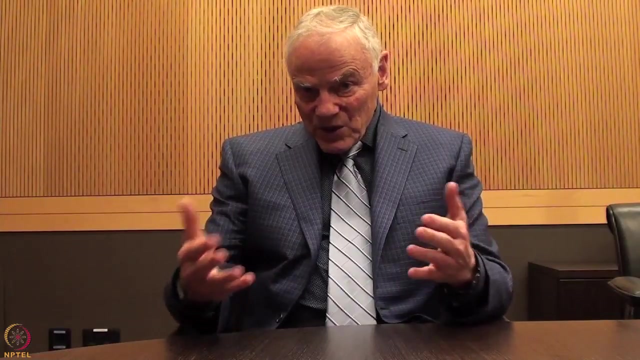 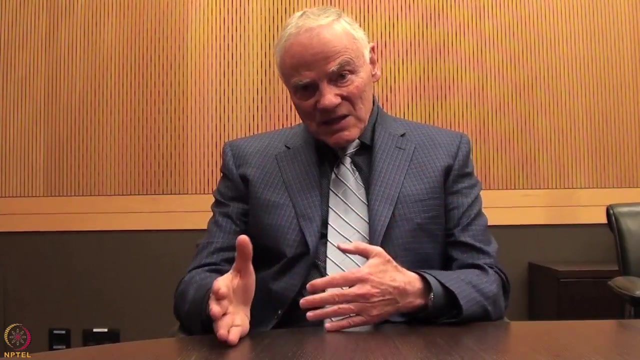 disease. but I think the really transformational possibility scientific wellness presents is that if you create a population of people that follow the scientific wellness program in a longitudinal manner and if that population begins to rate reach a certain critical level of thousands you you then begin to see wellness to disease transitions that you can use. the dense dynamic data cloud to get biomarkers to mark safety earliest transition for diabetes. and then you can begin to think about the systems, that technologies and systems-driven strategies that can be used to identify the disease-perturbed networks that will reveal candidates for creating drugs to reverse these diseases at their very earliest stage And if, for example, over a 20-year period, we can reverse all major diseases before they ever really manifest themselves as a disease and become irreversible, we'll save the health care system an enormous amount of money. In the US, for example, 86% of our enormous health care. 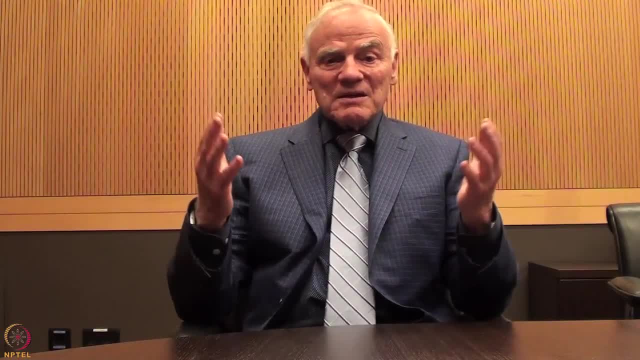 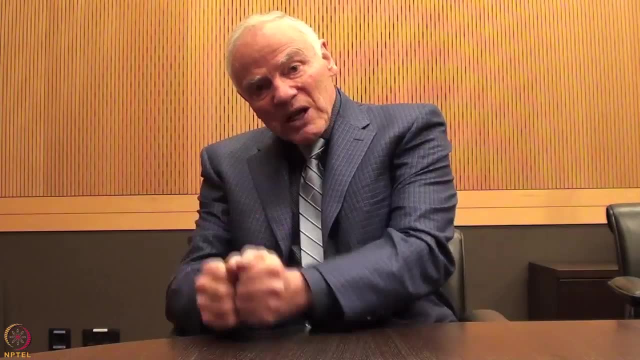 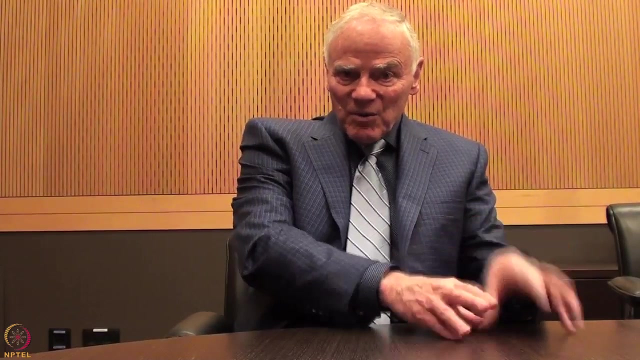 budget goes to chronic diseases. Suppose, in 20 years there are very few chronic diseases left. We've transformed a health care system that thinks only about disease to a health care system entirely focused on the disease. I'm optimizing wellness for their population. This is the opportunity that India has and I'd be. 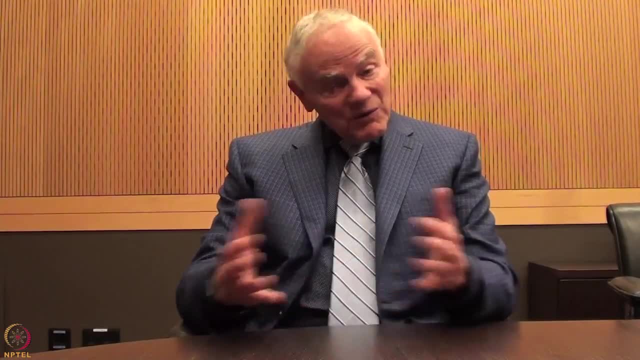 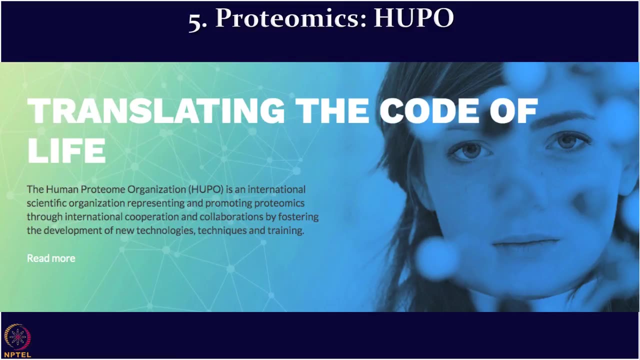 delighted to help you in that endeavor if you decide to make the commitment. So, finally, coming back to the proteomics, and the field of proteomics is now very well led with the efforts of Human Proteome Organization, which tagline is Translating the Code of Life. 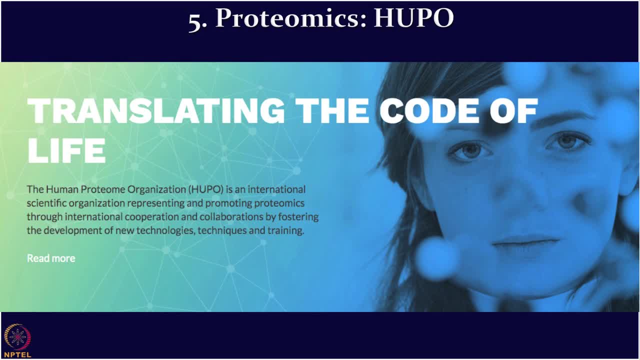 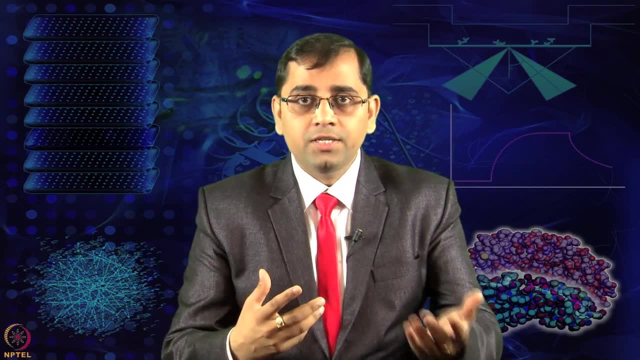 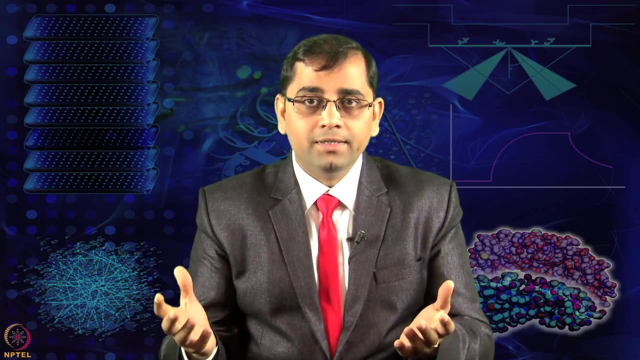 The idea is many scientists working in the field of proteomics and integrated omics- how to come together- will start sharing the data, will start sharing the ideas, exchange their various information, build collaboration and come forward for the big projects, And human proteome project is one of the. 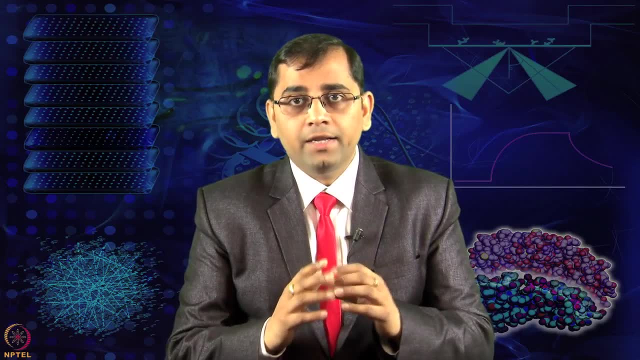 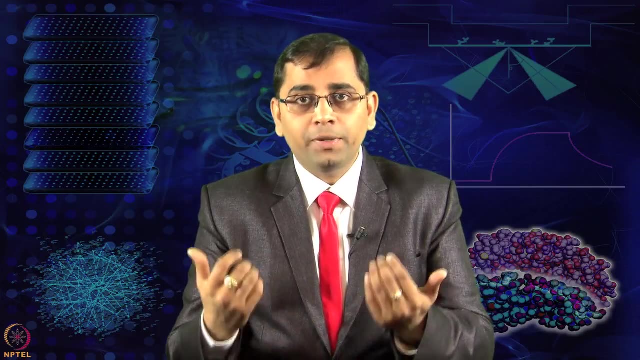 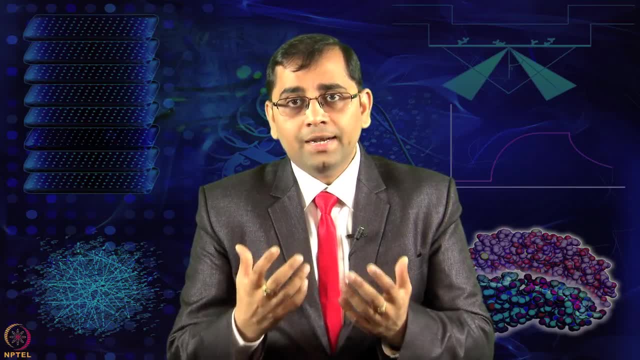 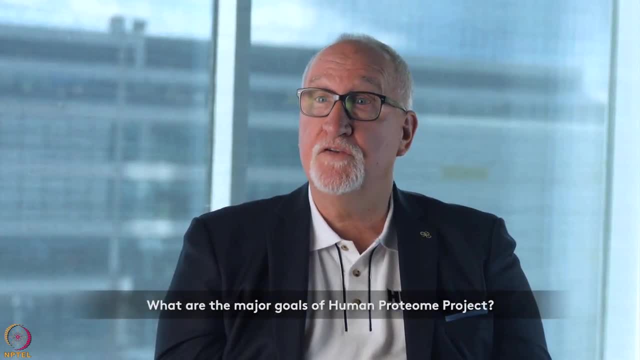 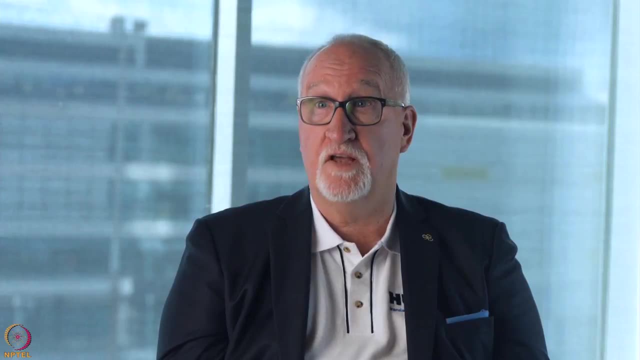 The human proteome project has two major goals. The first is to map the expression of the human genome, in terms of which proteins are made and which post-translational modifications are on those proteins that affect its activity, And the second is to springboard our discovery in COLIN. 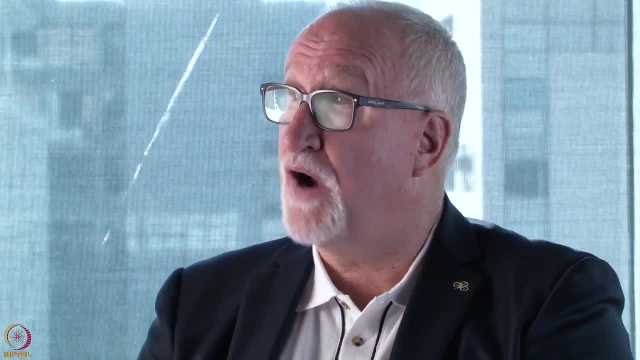 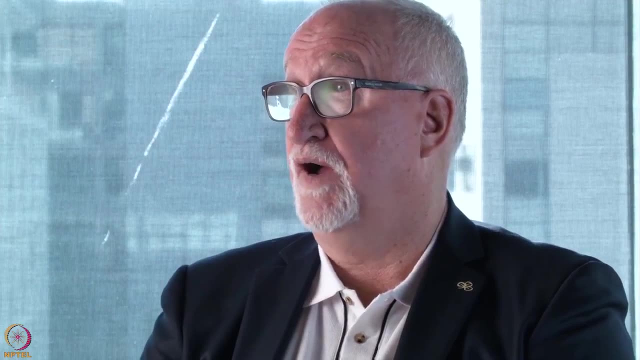 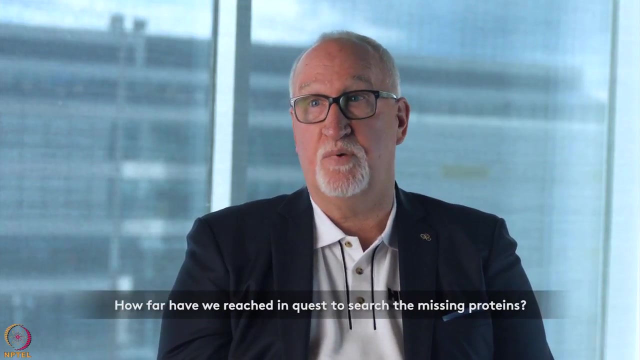 And the second is to springboard our discovery in COLIN, new drugs, discovery around biomarkers for human disease and an understanding of human health and wellness. One of the major activities of the Human Proteome Project has been to determine how many of those proteins 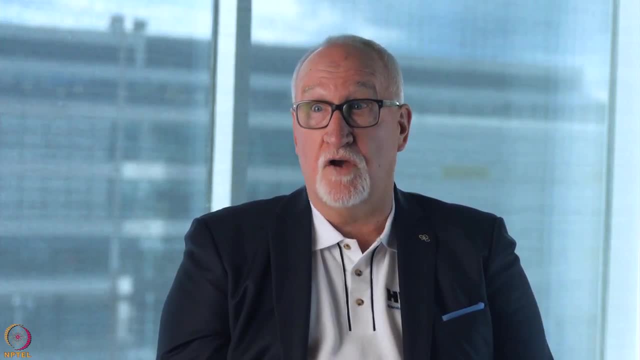 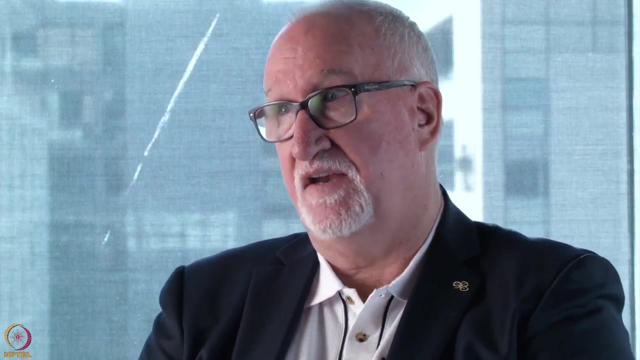 we've observed in human health and human disease. So far we've taken an approach that looks at about 85% of the total proteome content of the human proteome. But out of the 15% that's missing about 7% of them. we have some evidence for them. 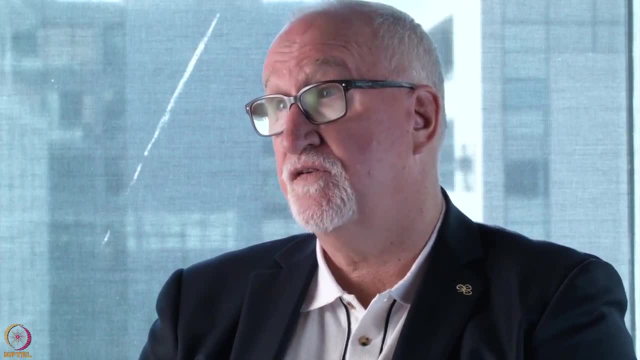 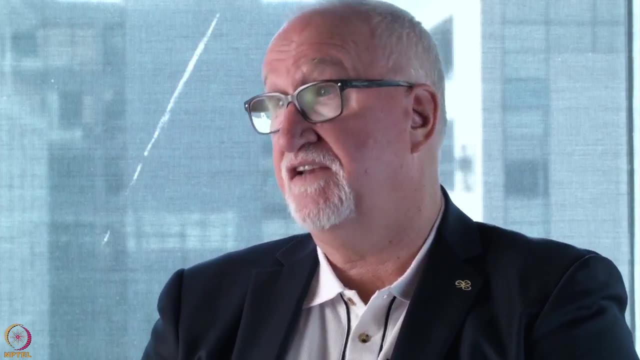 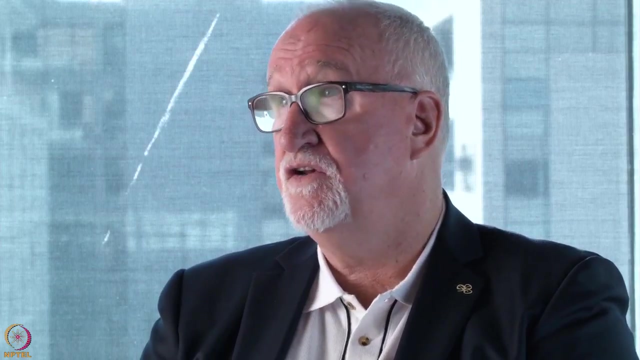 That's either mass spectrometry evidence or evidence that comes from other types of scientific experiments- biochemistry, physiology, pharmacology, genetics- But there are still about 1,000 proteins in the human proteome that we have absolutely no scientific evidence for their existence whatsoever. 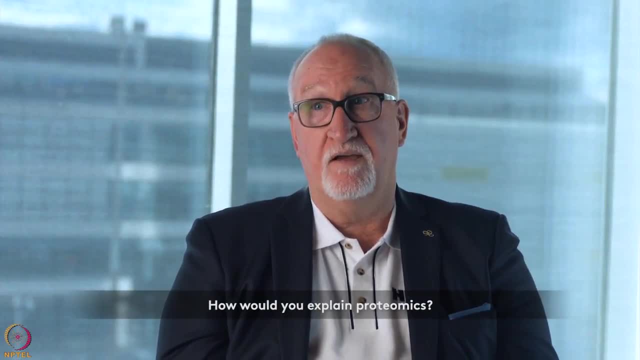 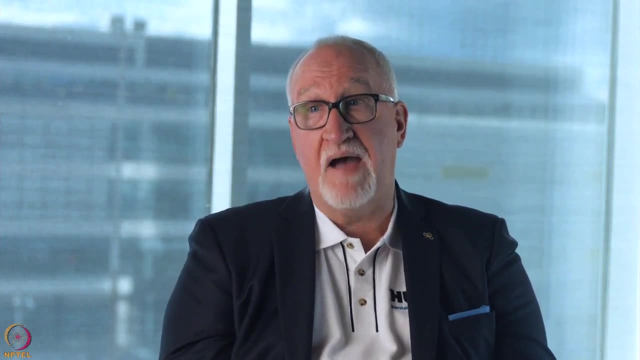 Proteomics is not a problem. It's not a word that everyone in the street knows. If I was to explain what proteomics was, it's effectively the protein complement or the machines that are made from the human genome, from the coding instructions, into something real. 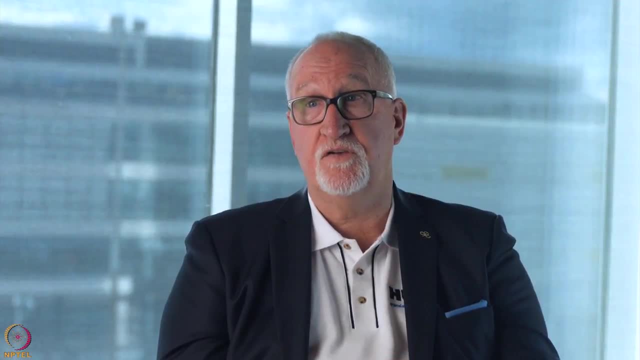 that makes a human body work. So the proteins are those things that are important in the machinery of life, in the reproduction of life and in the development of disease. That's why it's important for us to understand the proteins as well as the genes. 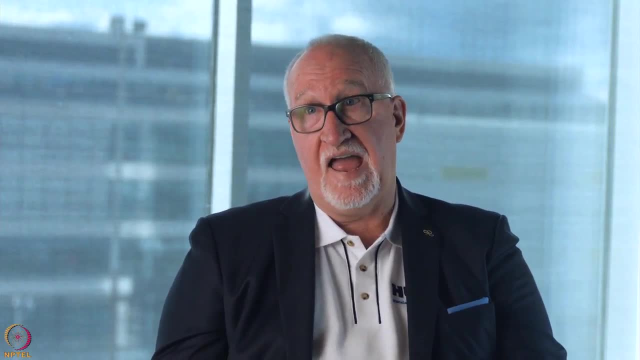 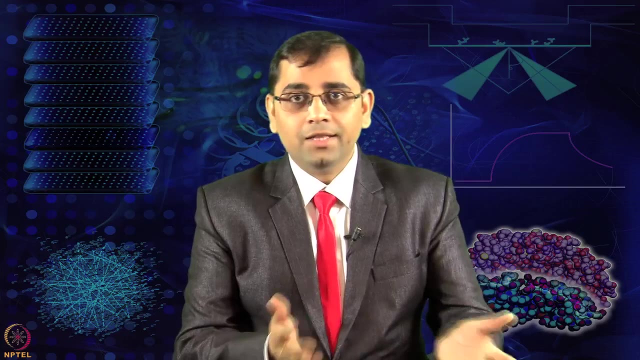 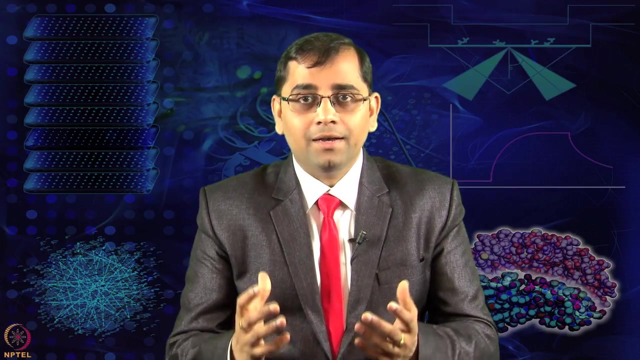 in order for us to understand human biology and how that goes awry in human disease. Additionally, it will be interesting to also listen the last three HUPO presidents, Mark Baker, Mike Schneider and Steven Pennington, and hear from their perspective. 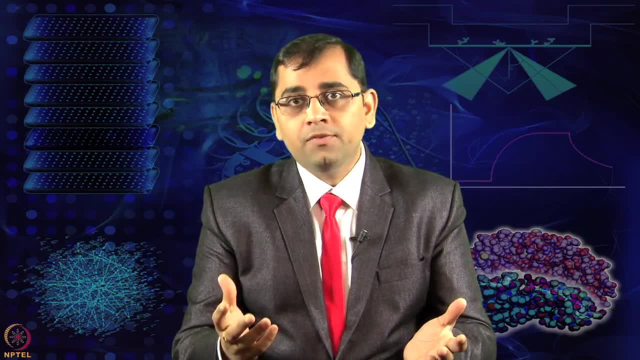 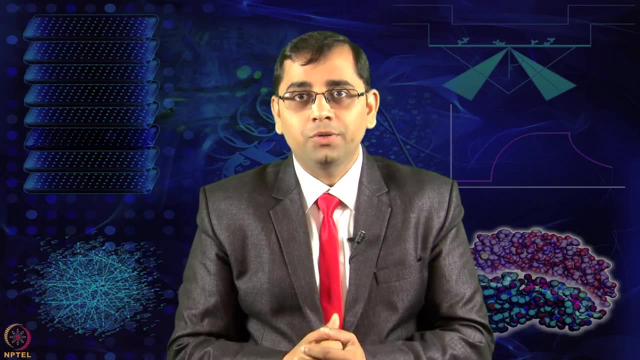 what proteomics and HUPO have achieved so far and what are their vision for the future guidelines for doing research in this area? I hope this will be interesting conversation for you to know the perspective of these leaders who are leading the field of proteomics. 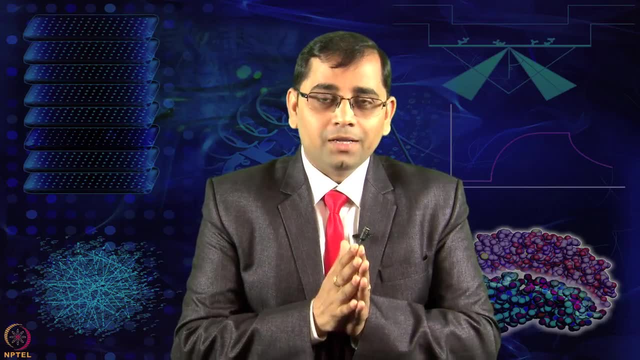 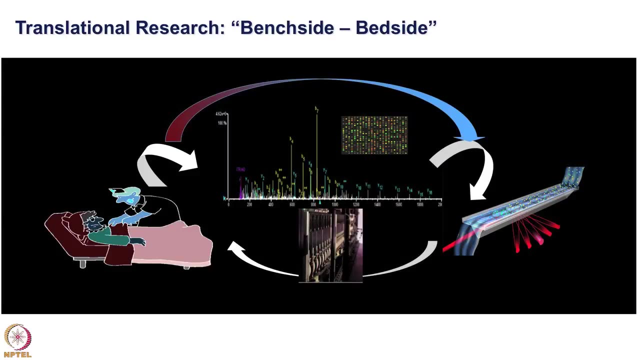 Okay, So finally, I'll stop here to show you this slide, which is a motivation for many people working in this field of omics and life sciences, where a lot of you know the actual problem. we want to find the cues and the mechanism. 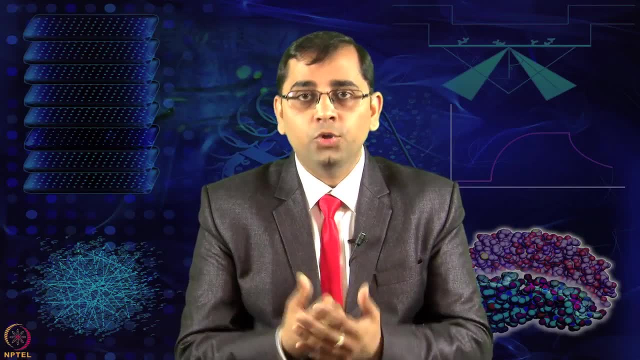 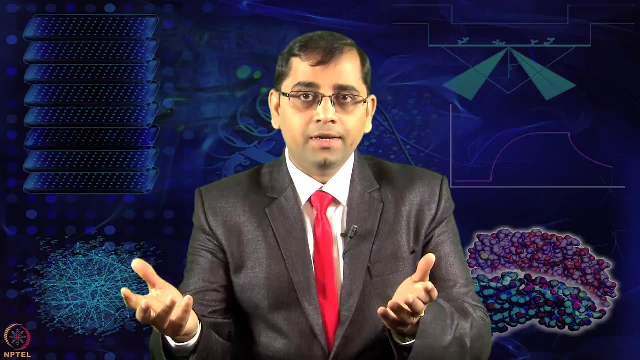 and the leads, understanding them at the omics level, at the molecular level, and then want to translate our bench side. for example, We want to translate our findings to the bedside for the actual patient care or for the actual biological system to really make impact of that. 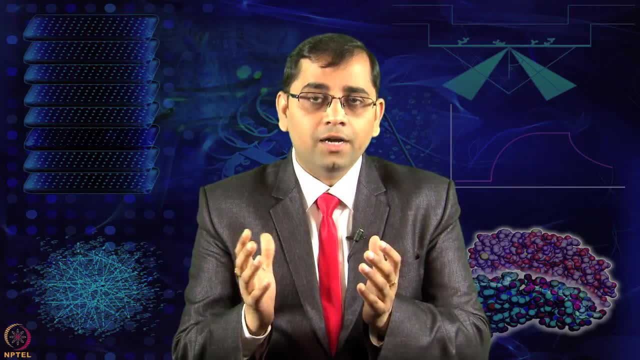 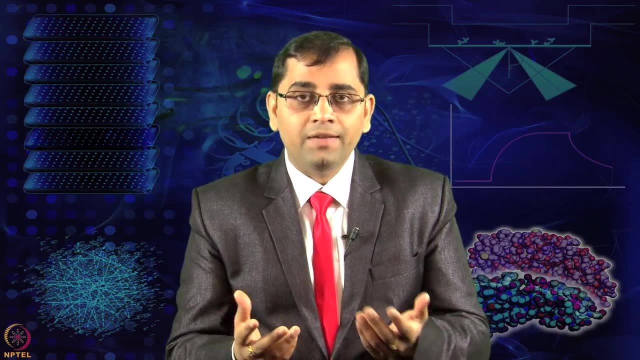 And that's where all of this understanding, all of these technologies are really going to help us to achieve that major goal. I hope you this whole course, the different type of live sessions, different demonstrations, were helpful for you to appreciate the power.